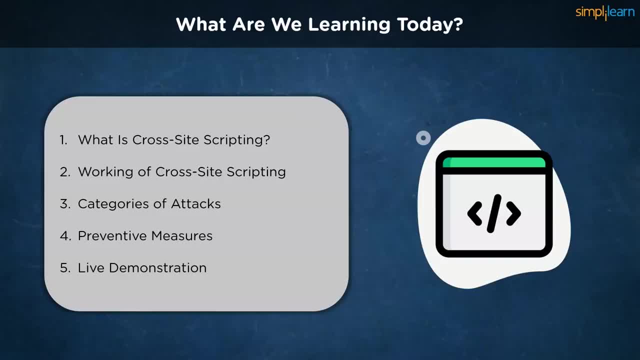 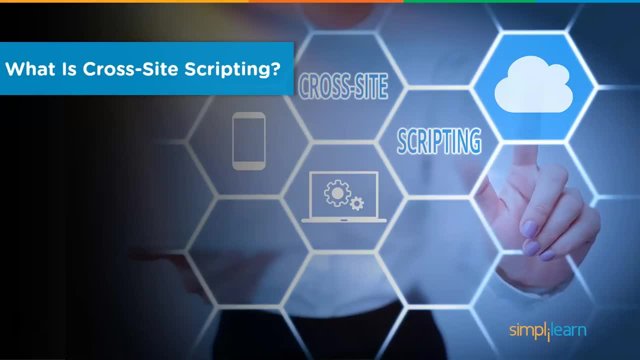 number of attacks and the number of attacks that can be inflicted by a victim. In this video, we will learn about the cross-site scripting attack and how a simple line of code can open up vulnerabilities if not configured correctly. Let's start by learning about cross-site scripting from a layman's perspective. 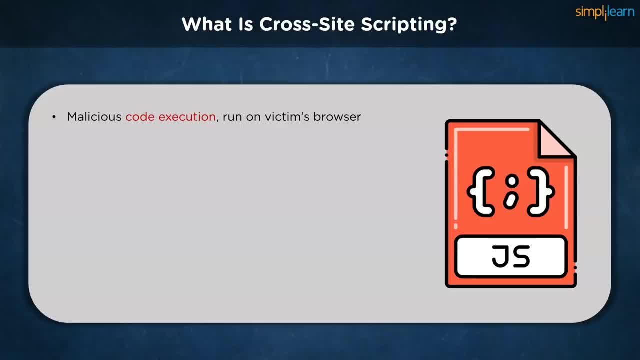 Cross-site scripting, also known as XSS, is a type of code injection attack that occurs on the client side. The attacker intends to run harmful scripts in the victim's web browser. by embedding malicious code in a genuine webpage or online application, The real attack takes. 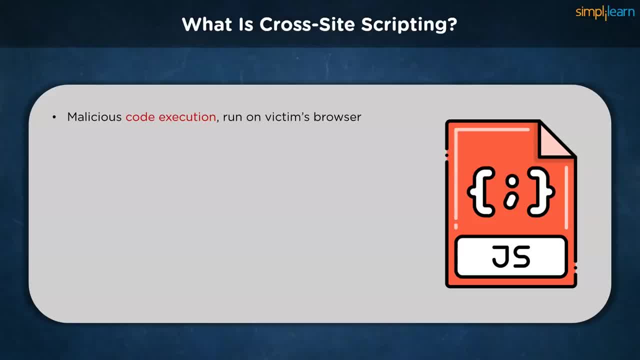 place when the victim hits the malicious, code-infected web page or online application. The web page or application serves as a vehicle for the malicious script to be sent to the user's browser. Forums, message boards and online pages that enable comments are vulnerable. 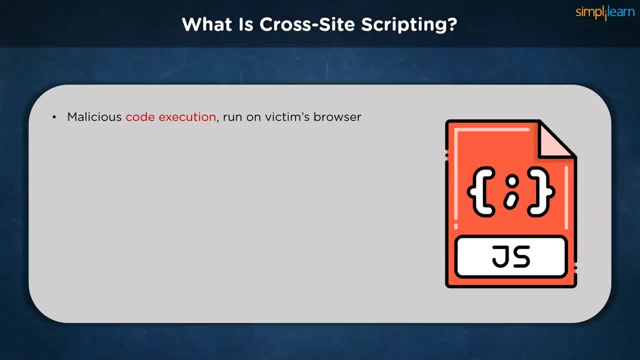 vehicles that are frequently utilized for cross-scripting assaults. A web page or web application is vulnerable to XSS if the output it creates contains unsanitized user input. The victim's browser must then parse this user input In VBScript, ActiveX, Flash and even CSS. cross-site scripting attacks are conceivable. 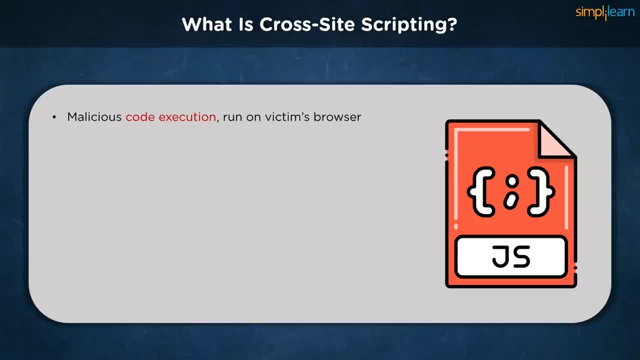 They are nevertheless most ubiquitous in JavaScript, owing to the fact that JavaScript is most important to most browser experiences nowadays. The main purpose of this attack is to steal the other user's identity, be it via cookies, session tokens and other information. In most of the cases, this attack is being used. 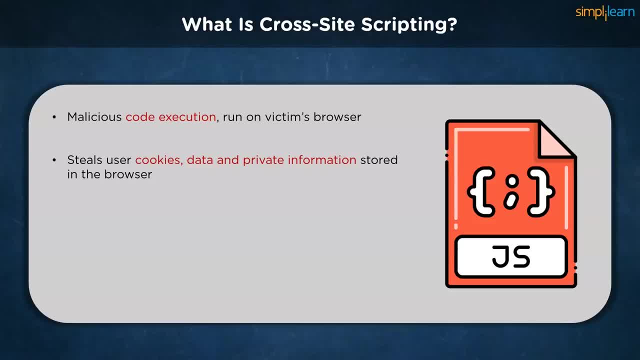 to steal the other person's cookies. As we know, cookies help us to log in automatically. Therefore, with the stolen cookies, we can log in with other identities, And this is one of the reasons why this attack is considered as one of the riskiest attacks. It can be performed with different client-side programming. 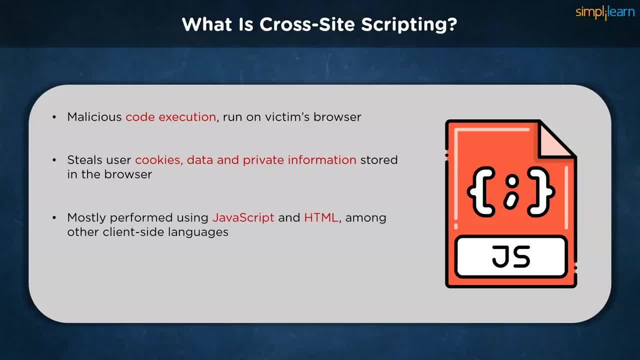 languages as well. Cross-site scripting is often compared with similar client-side attacks, as client-side languages are mostly being used during this. However, an XSS attack is considered riskier because of its ability to damage even less vulnerabilities. Most often, this attack is performed with JavaScript and HTML. 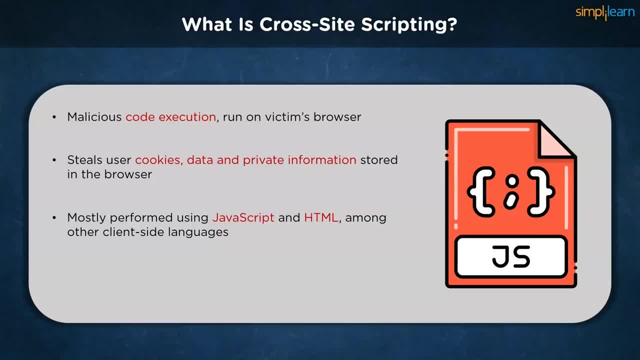 JavaScript is a programming language that runs on web pages inside your browser. The client-side code adds functionality and interactivity to the web page and is used extensively on all major applications and CMS platforms. Unlike server-side languages such as PHP, JavaScript code runs inside your browser and cannot impact the website for other visitors. 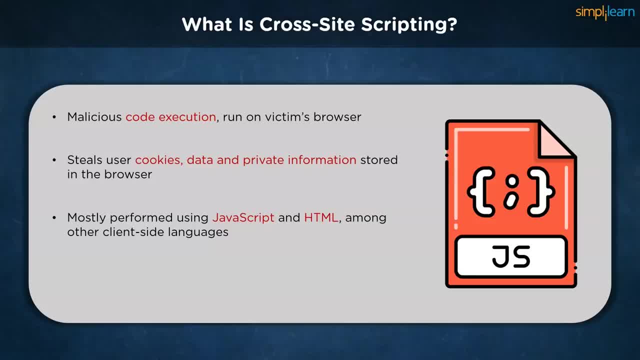 It is sandboxed to your own navigation. It is also a very powerful tool to use for the use of your own browser and can only perform actions within your own browser window. While JavaScript is client-side and does not run on the server, it can be used to interact. 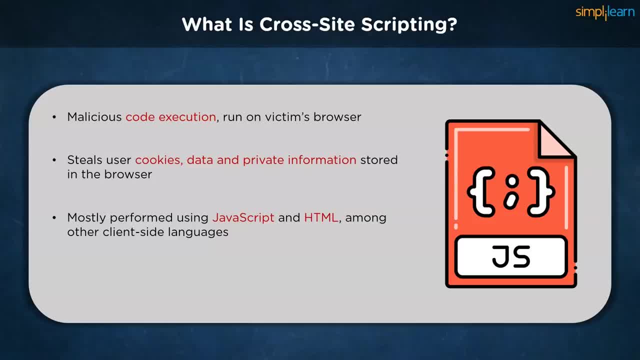 with the server by performing background requests. Attackers can then use these background requests to add unwanted spam content to a web page without refreshing it. They can then gather analytics about the client's browser or perform actions asynchronously. The manner of attack can range in a variety of ways. 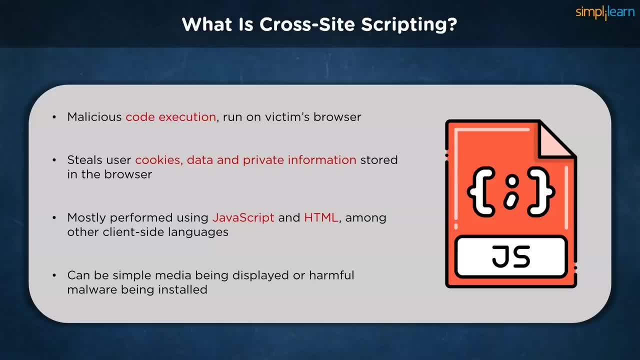 It can be a single link which the user must click on to initiate a JavaScript piece of code. It can be used to show any piece of images that can be later used as a front-end for malicious code being installed as malware. With the majority of internet users unaware of how metadata works or the ways in which 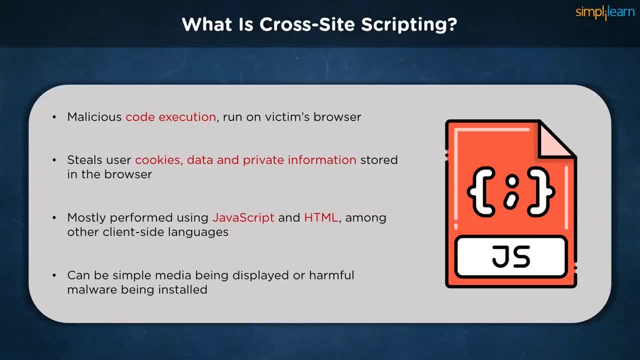 web requests are called. the chances of victims clicking on and redirecting links is far too high. Cross-site scripting can occur on the malicious script executed at the client's site using a fake page or even a form that is displayed to the user. 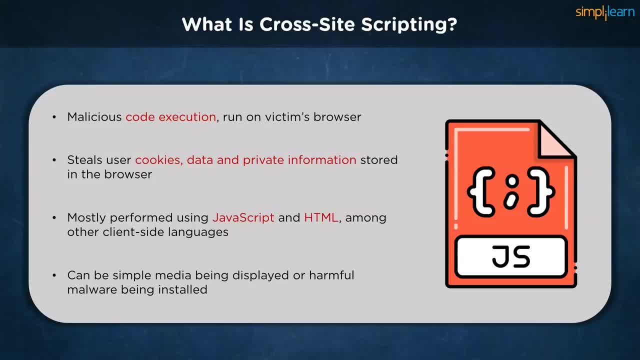 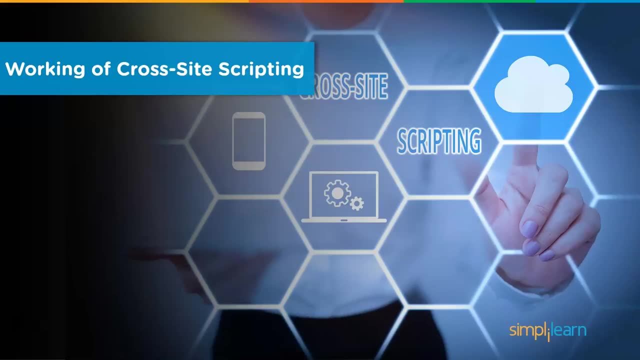 On websites with displayed advertisements, malicious emails can also be sent to the victim. These attacks occur when the malicious user finds the vulnerable parts of the website and sends it as appropriate malicious input. Now that we understand the basics of cross-site scripting, let us learn more about how this 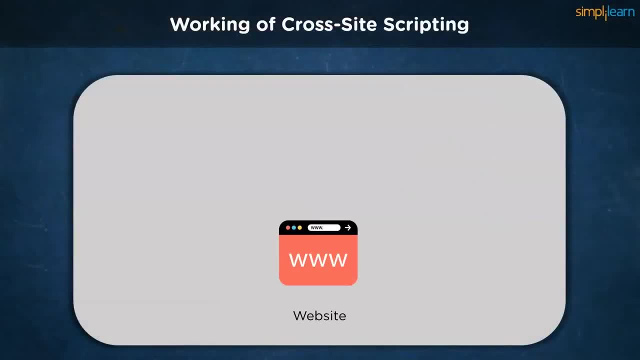 kind of attack works Now? first place, we have the website or the web browser which is used to show content to the victim, or which is the user in our case. Whenever the user wants to grab some content from the website, the website asks the data. 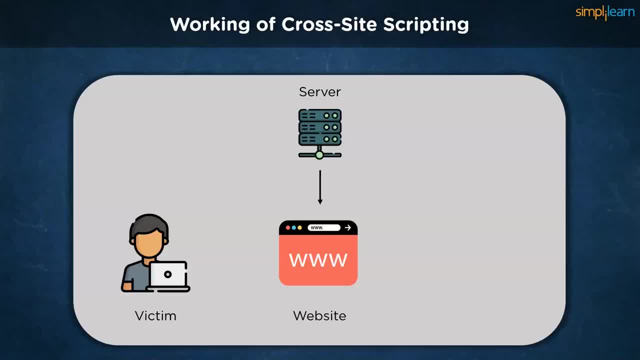 from the server. The server provides this information to the website and the web browser, which ultimately resists the victim. How the hacker comes into play here: It passes on certain arguments to the web browser, which can be then forwarded back to the server or to the user at hand. 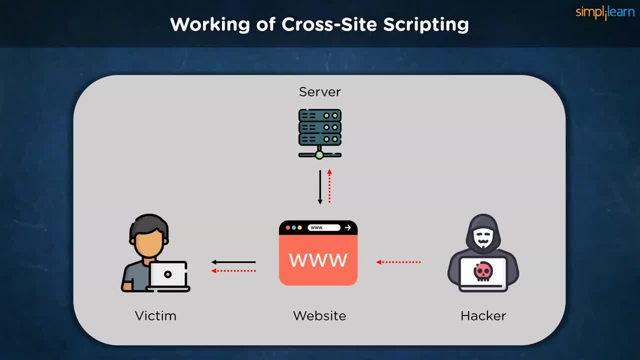 The entire cross-site scripting attack vector means sending and injecting malicious code or script. Attack can be performed in different ways Depending on the type of attack. the malicious script may be reflected on the victim's browser, but stored in the database and executed every time when the user calls the appropriate. 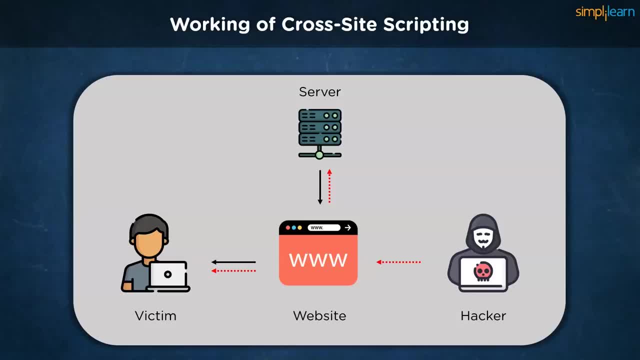 function. The main reason for this attack is inappropriate user's input validation, where the malicious input can get into the output. A malicious user can enter a script which will be injected onto the website's code. Then the browser is not able to know if the executed code is malicious or not. 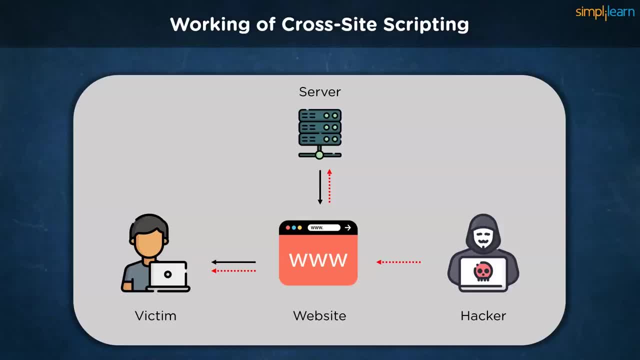 Therefore, this malicious script is being executed on the victim's browser or any faked form, if that is being displayed for the users. There are many ways to trigger an XSS attack. For example, the execution could be triggered automatically when the page loads or when 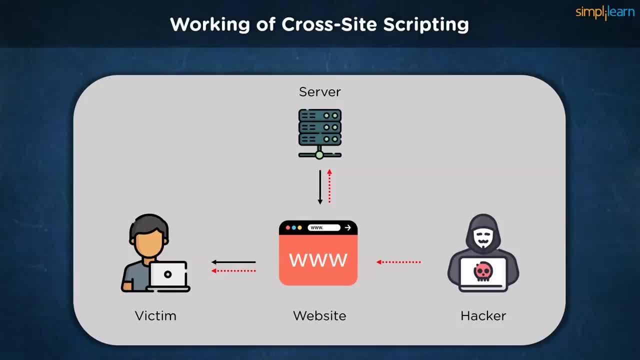 a user hovers over specific elements of the page, like hyperlinks. Potential consequences of cross-site scripting attacks include capturing keystrokes of a user, redirecting a user to malicious websites, running web browser based exploits and even using malicious code to hack the user's account. 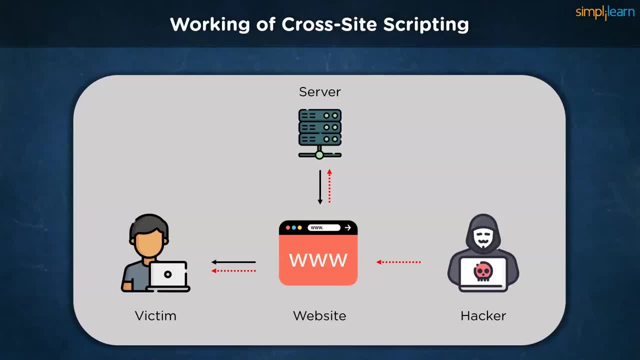 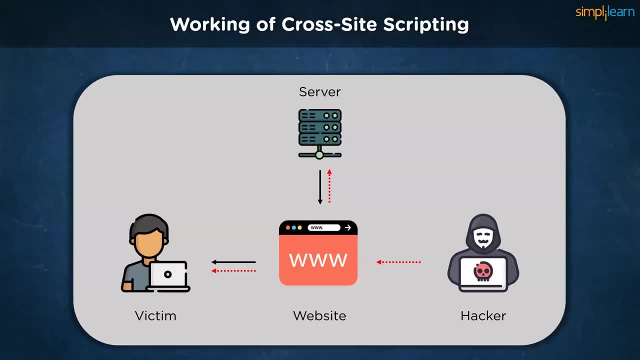 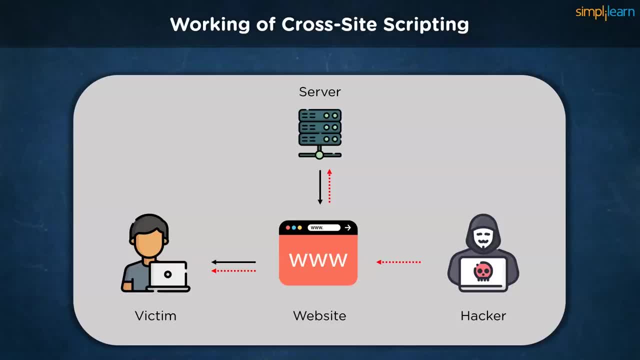 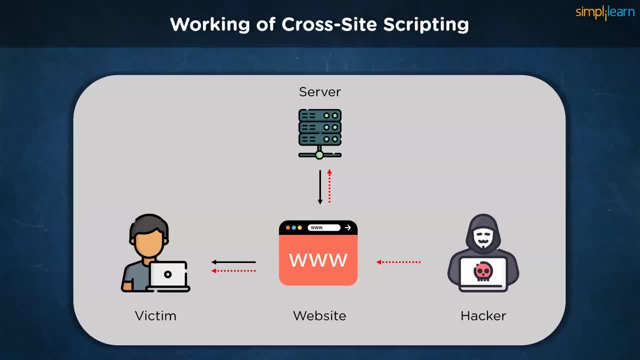 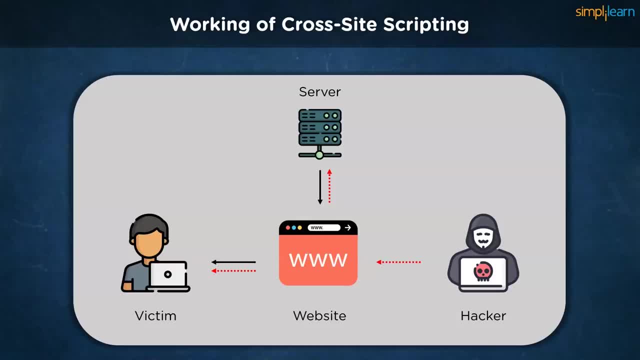 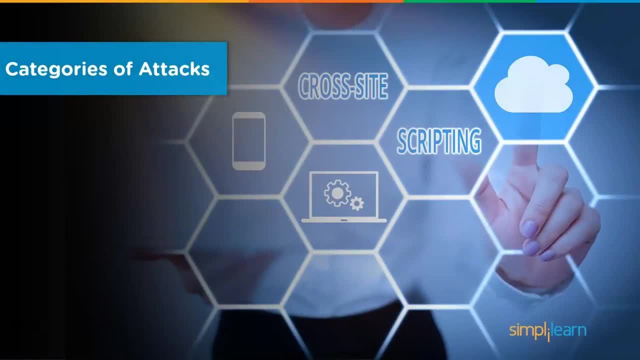 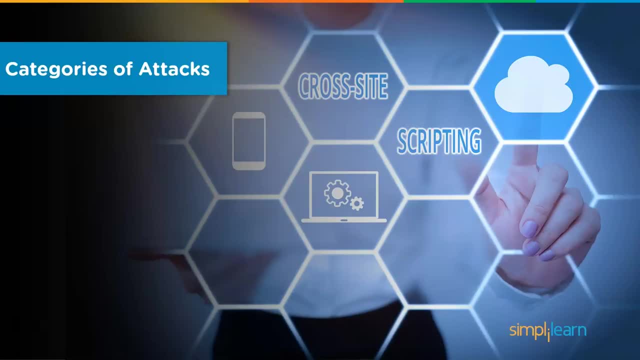 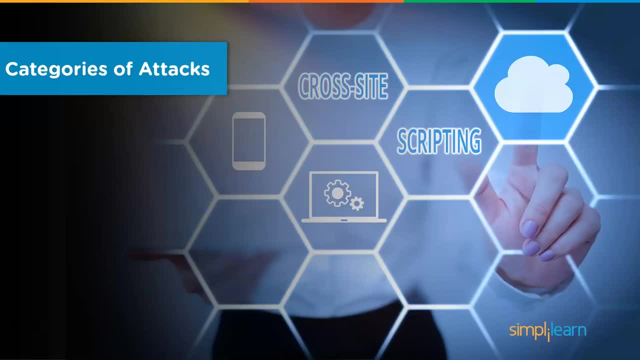 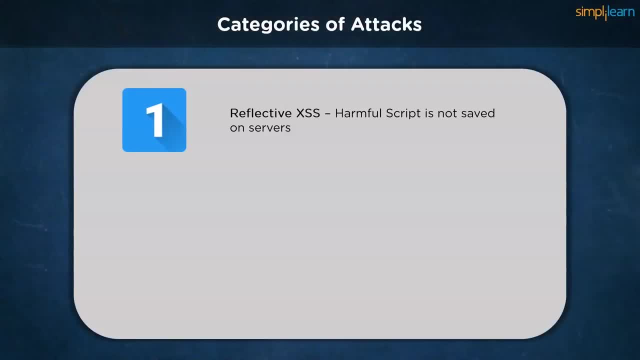 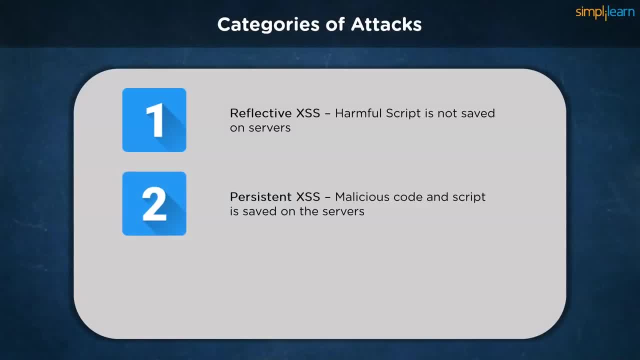 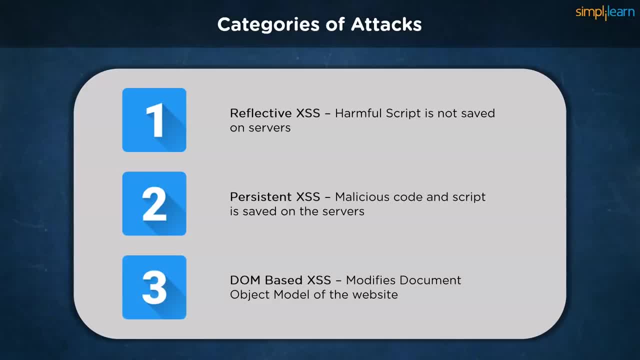 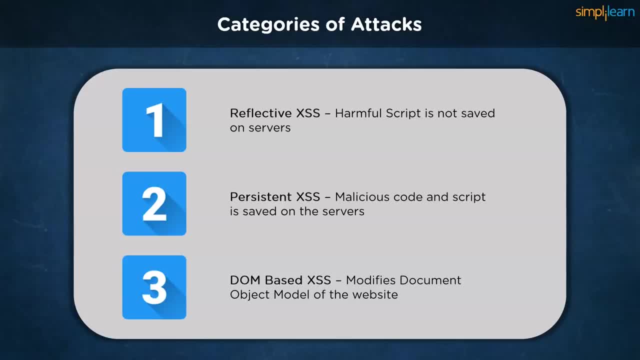 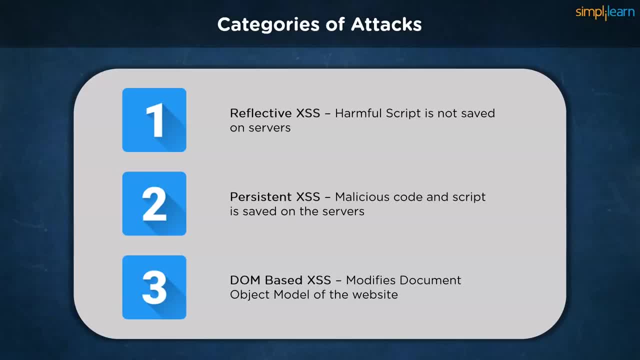 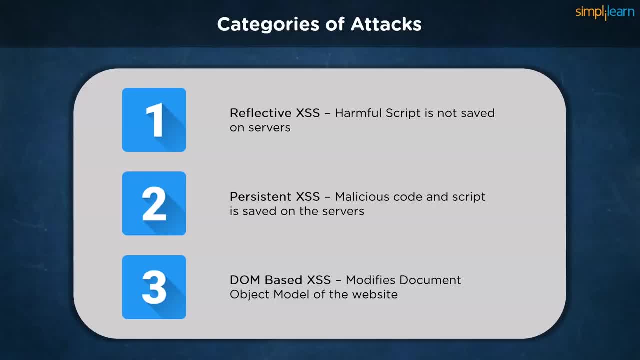 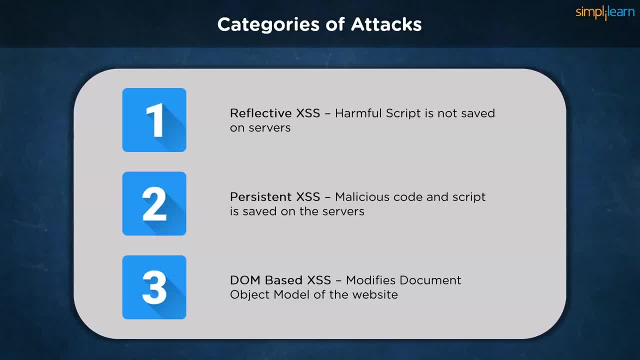 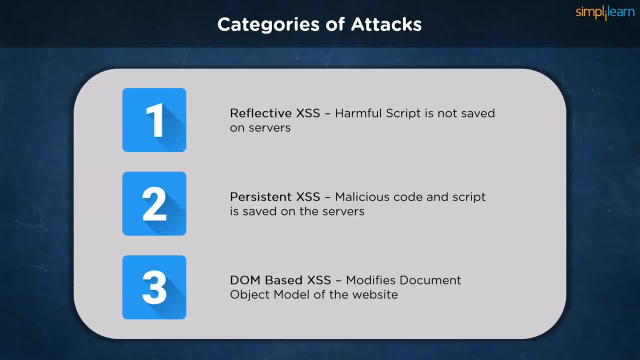 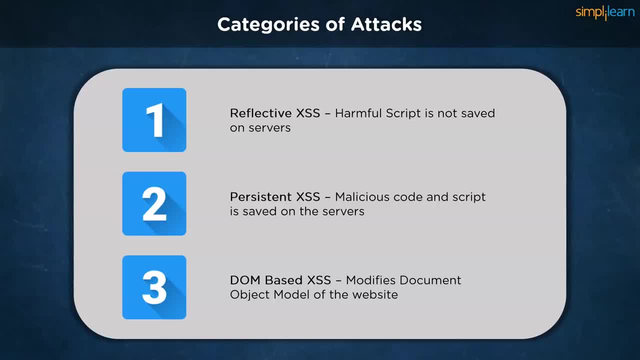 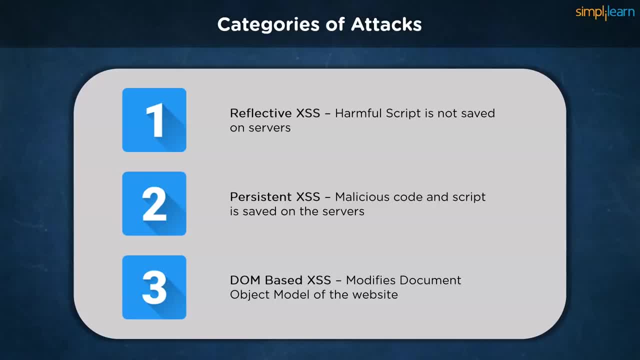 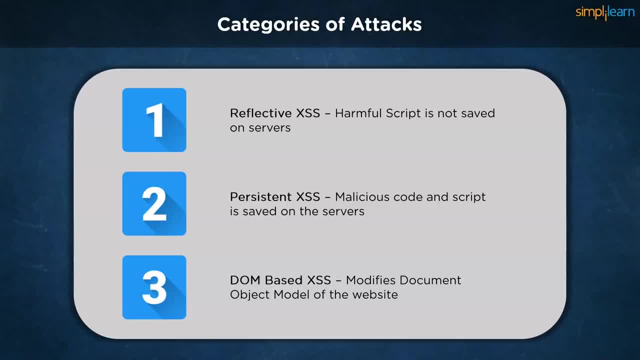 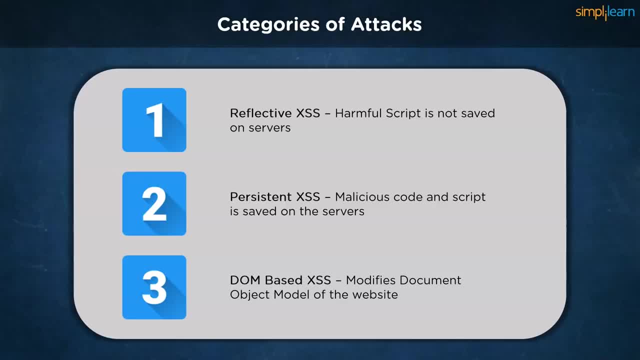 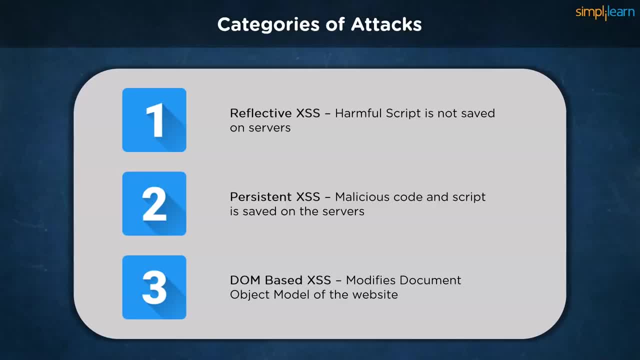 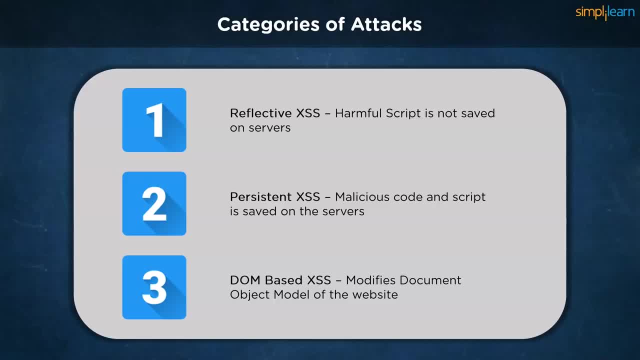 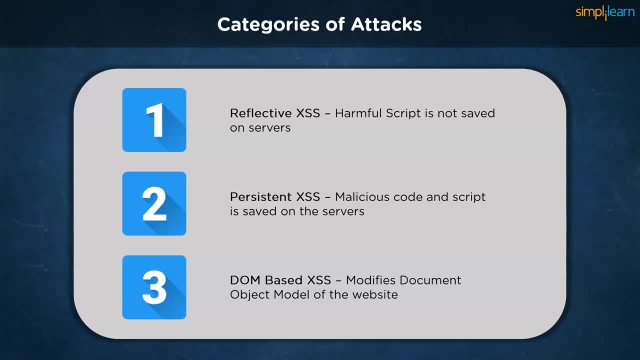 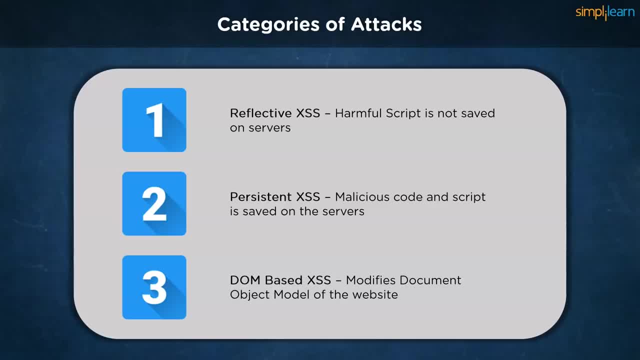 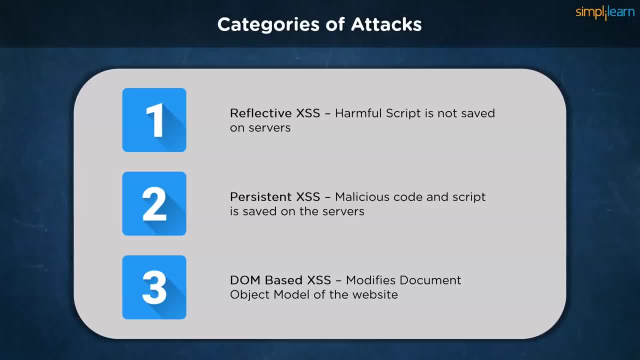 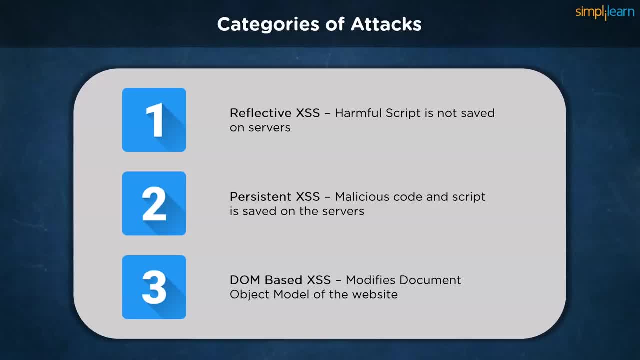 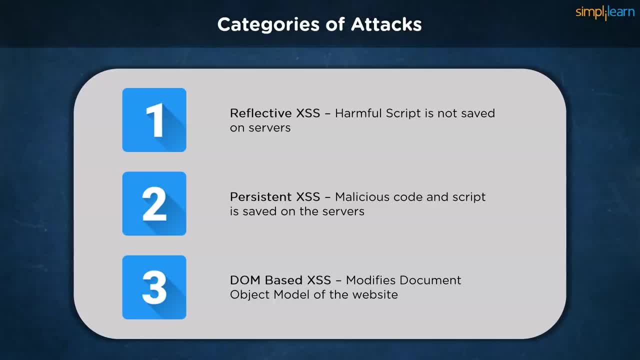 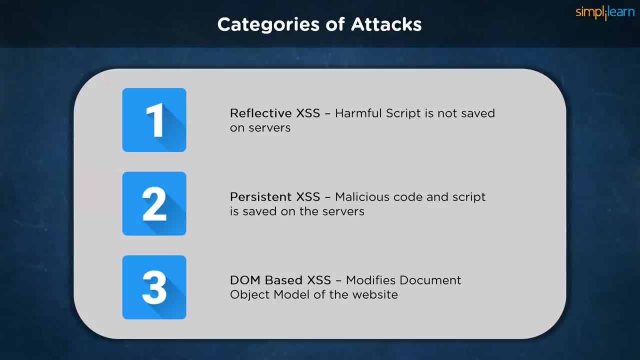 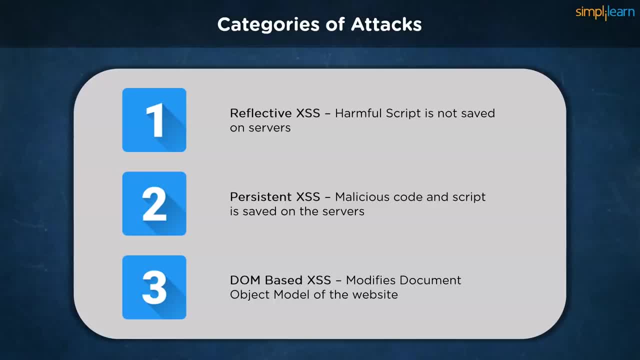 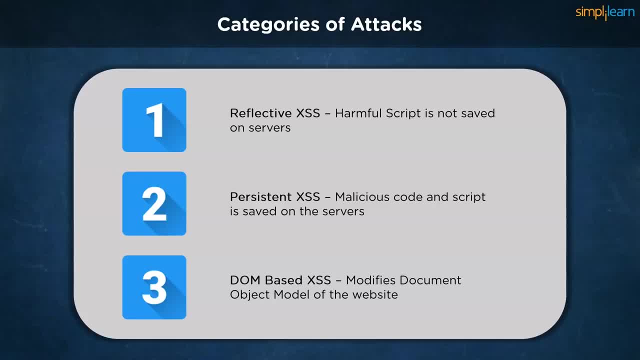 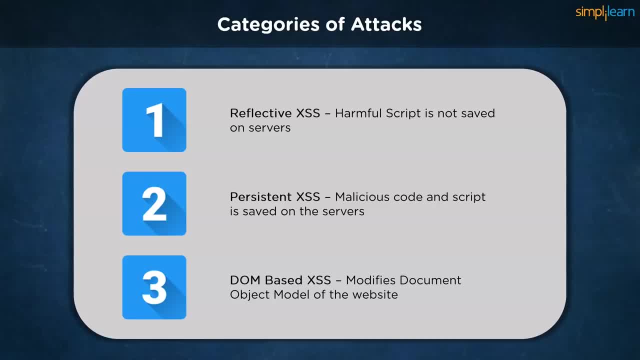 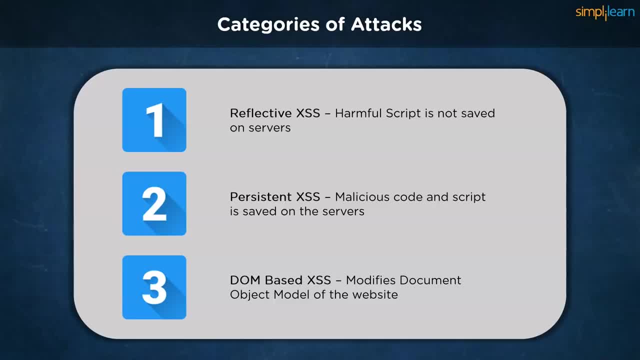 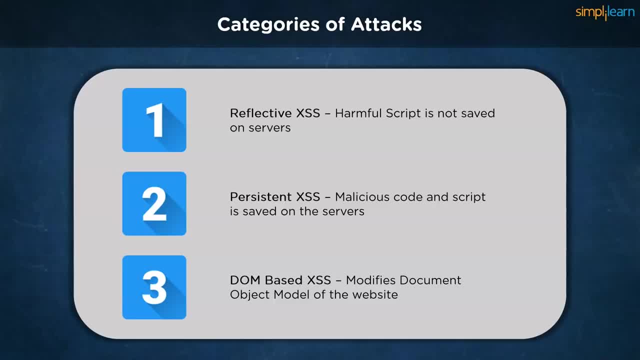 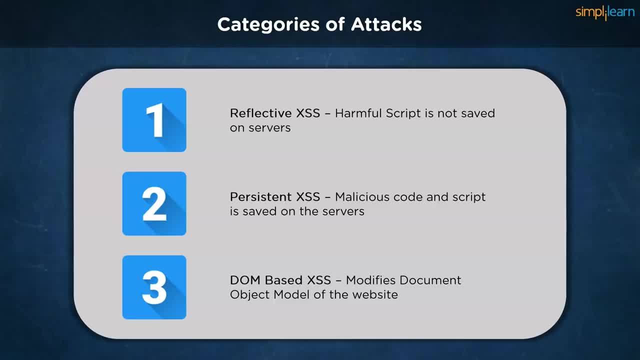 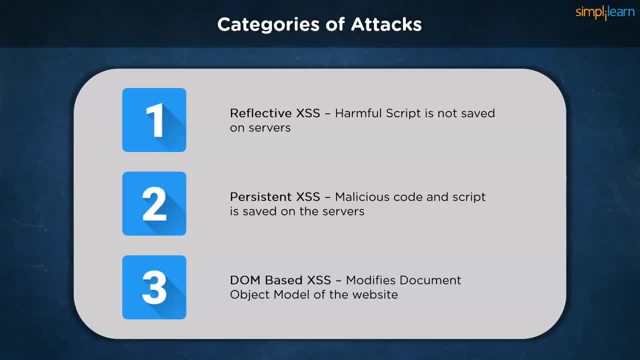 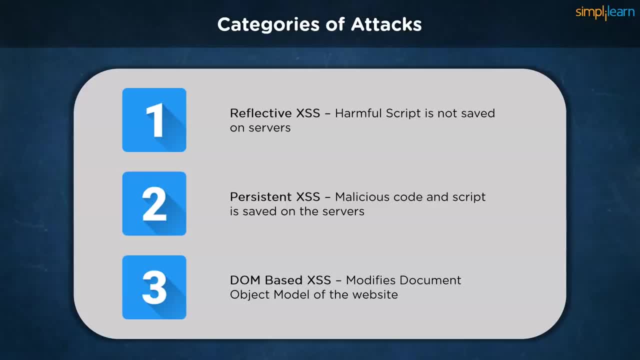 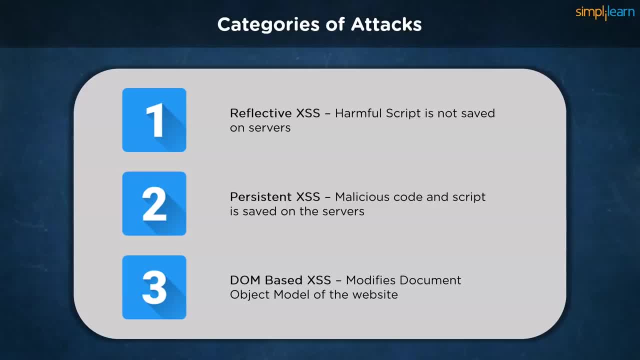 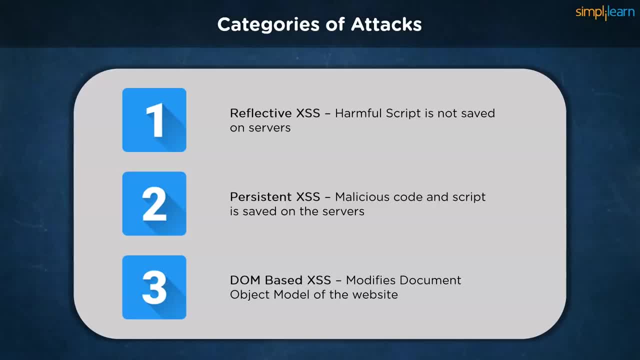 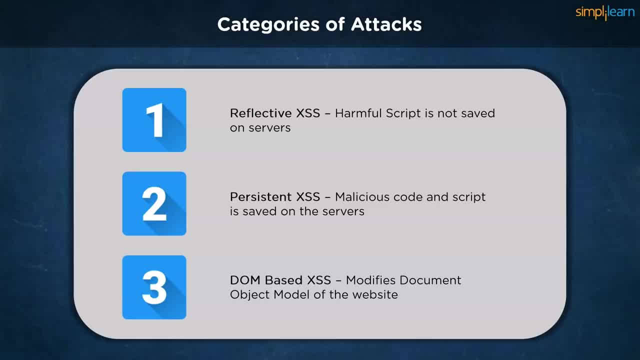 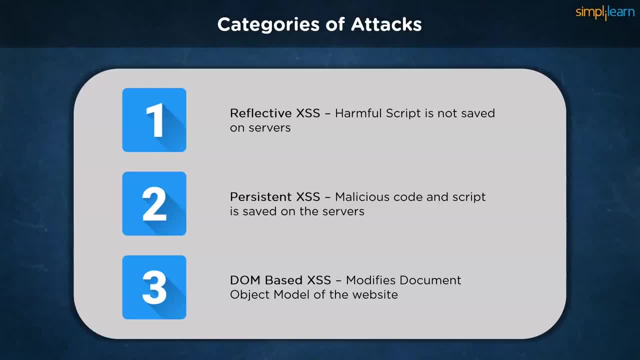 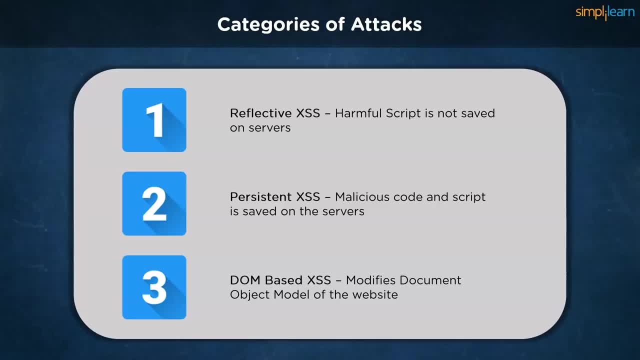 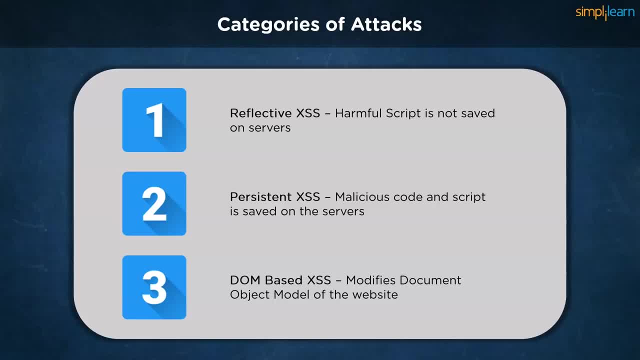 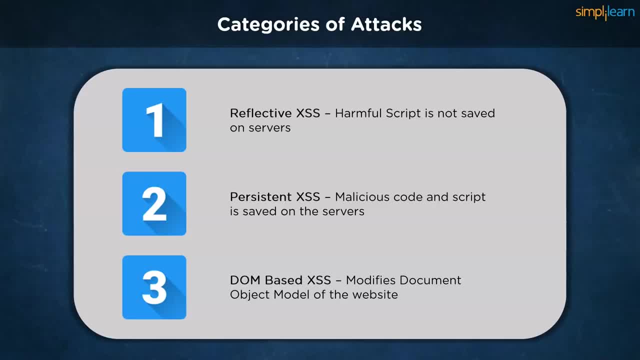 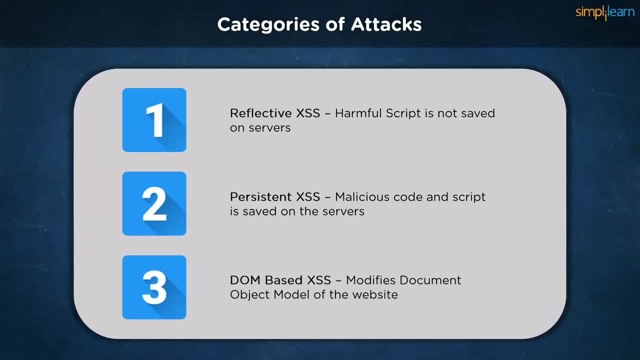 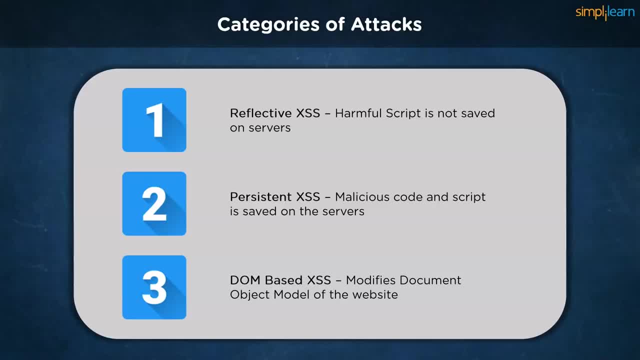 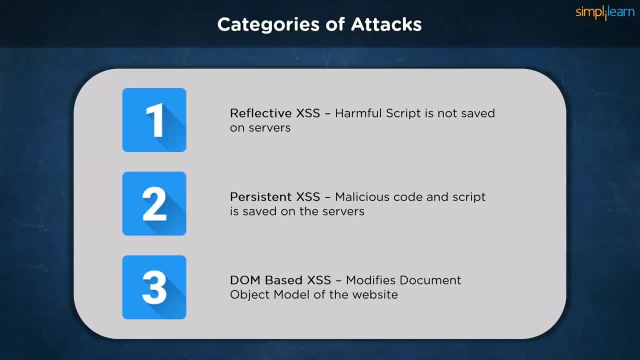 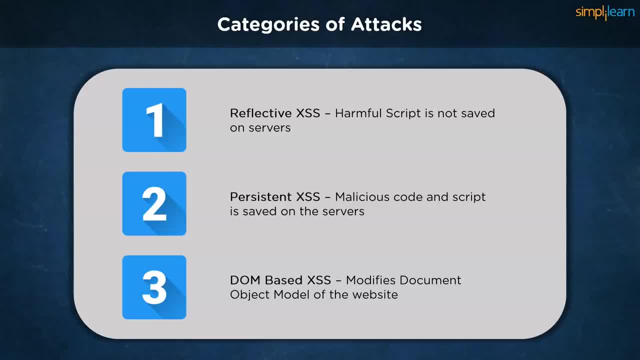 The user can then use the malicious script to hack. the user's account is now being delivered to all users visiting the web application and they, for example, able to gain access to the user session cookies. In this attack, the script is permanently stored in the web app. The users visiting the app after the. 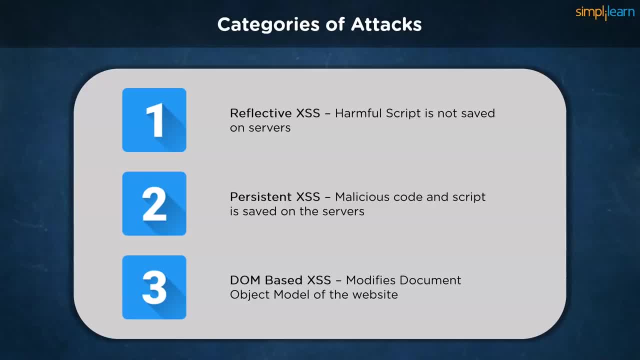 information, retrieve the script. The malicious code then exploits the flaws in the web application and the script, and the attack is visible on the server side or to the app owner as well. The third variant is DOM based cross-site scripting attacks. This type of attack occurs when the DOM environment is 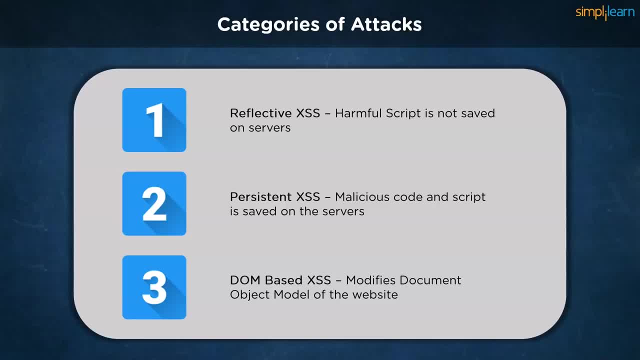 being changed, but the client-side code does not change. When the DOM environment is being modified in the victims browser, the client-side code executes differently. In order to get a better understanding of how XSS DOM attack is being performed, let us analyze the following example. If there is a website, 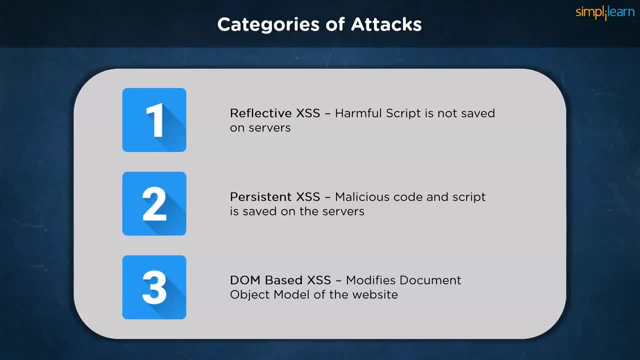 called textincom. we know default is a parameter. Therefore, in order to perform XSS DOM attack, we should send a script as parameters. A DOM based access S attack may be successfully executed even when the server does not embed any malicious code into the webpage by using a flaw in the JavaScript executed in the browser. For 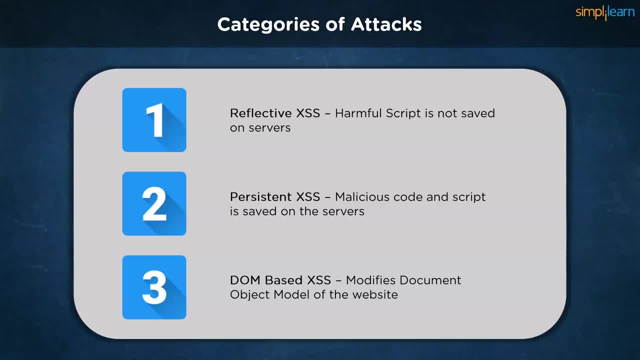 example, if the client side JavaScript modifies the DOM tree for the webpage, it can be based on an input field or the get parameter, without validating the input. This allows the malicious code to be executed. The malicious code exploits flaws in the browser on the user side and the script, and the attack is not necessarily. 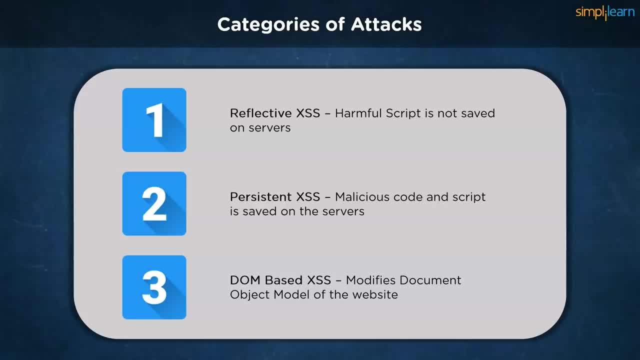 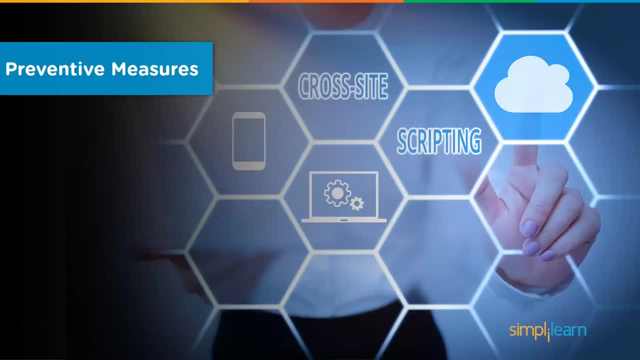 visible on the server side or to the app owner. By now, it is clear that cross-site scripting attacks are difficult to detect and even tougher to fight against. There are, however, plenty of ways one can safeguard against such attacks. Let's go through some of these preventive measures. 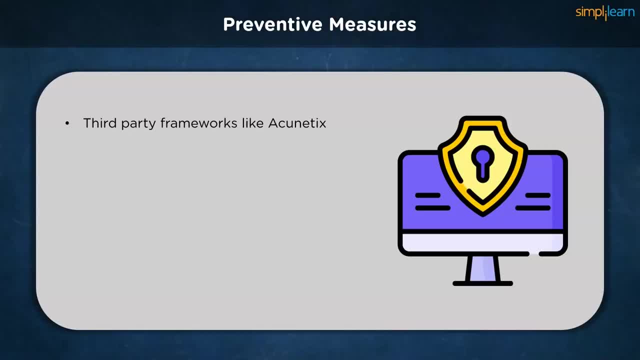 Like mentioned earlier, XSS attacks are sometimes difficult to detect. However, this can be changed if you get some external help. A way to prevent XSS attacks is using automated testing tools like Crashtest Security Suite or Acunetix Security Suite. 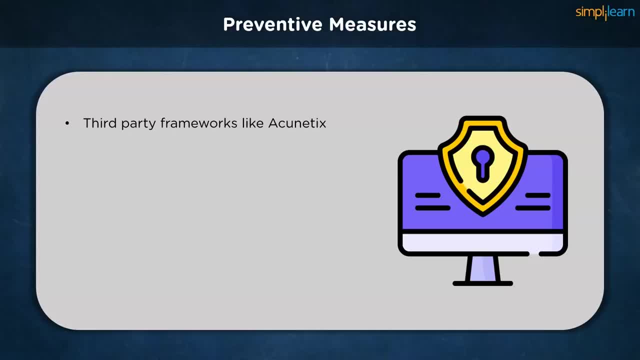 Still, manual testing is highly time-consuming and costly, and therefore not possible to be done for every iteration of your web application. Consequently, your code shouldn't be untested before any release. Using automated security is a good idea. With automated security, you can scan your web application for cross-site scripting and 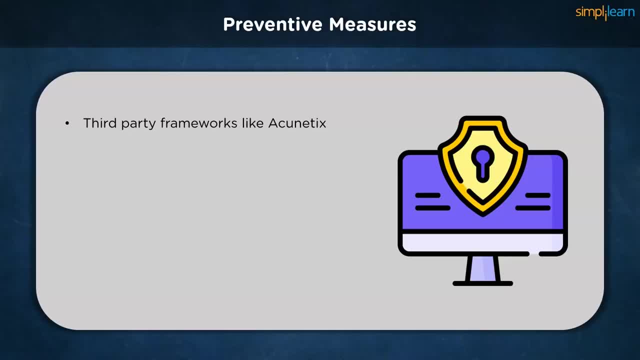 other critical vulnerabilities before every release. This way, you can ensure that your web application's live version is still secured whenever you alter or add a feature. Input fields are the most common point of entry for XSS attack scripts. Therefore, you should always screen and validate any information input into data fields. 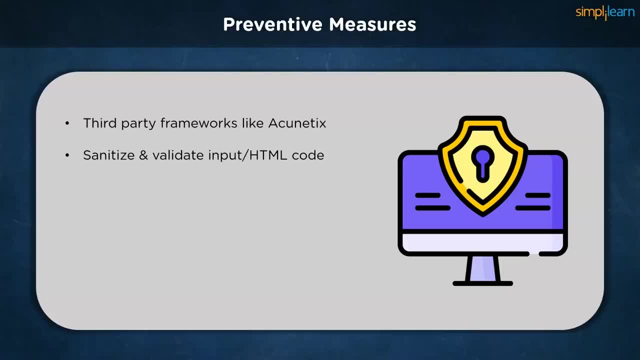 This is particularly important if the data will be included as HTML output. This can be used to protect against reflected XSS attacks. Validation should occur on both the client side and server side. as an added precaution, This helps validating the data before it's being sent to the servers and can also protect 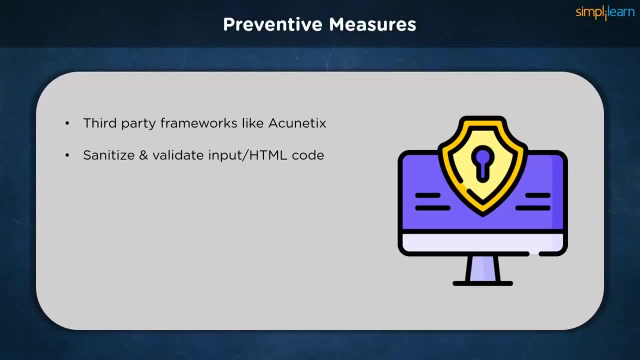 against persistent XSS scripts. This can be accomplished using JavaScript. XSS attacks only appear if any user input is being displayed on the web page. Therefore, try to avoid displaying any untrusted user input if possible. If you need to display user data, restrict the places where the user input might appear. 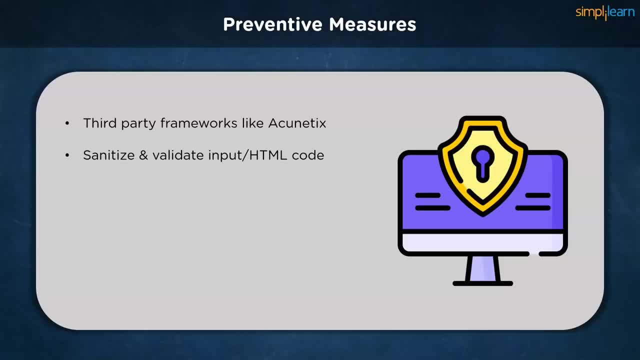 Any input displayed inside a JavaScript tag or a URL shown on the site is much more likely to be exploited than the input that appears inside a division or a span element inside the HTML body. Protecting against XSS vulnerabilities typically requires properly escaping user-provided data. 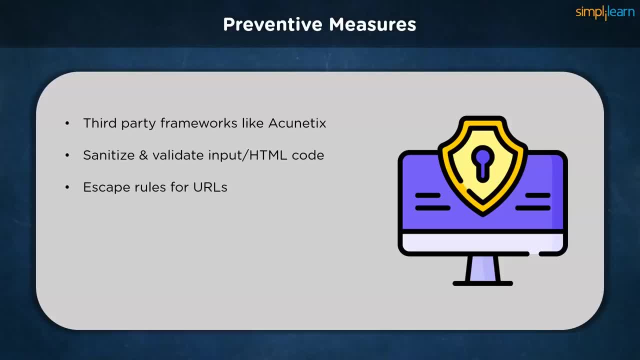 that is placed on the page, Rather than trying to determine if the data is user-provided and could be compromised. always play it safe and escape data, whether it is user provided or not. Unfortunately, because there are many different rules for escaping, you still must choose. 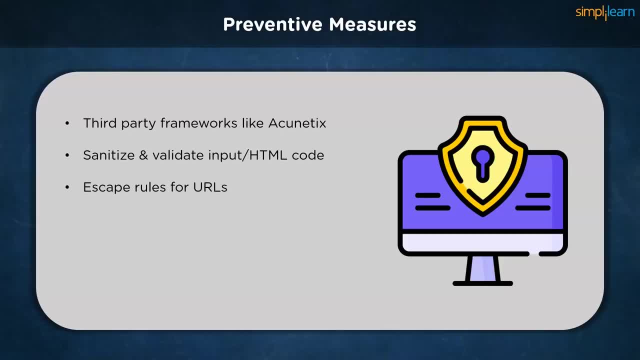 the proper type of escaping before settling on a final code. Encoding should be applied directly before user-controllable data is written to a page, because the context you're writing into determines what kind of encoding you need to use. For example, values inside a JavaScript string require a different type of code layer inside. 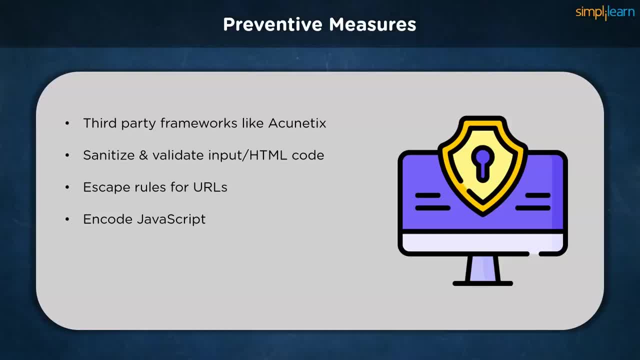 a JavaScript string of escaping to those in an HTML context. Sometimes you'll need to apply multiple layers of encoding in the correct order. For example, to safely embed user input inside an event handler. you need to deal with both JavaScript context and the 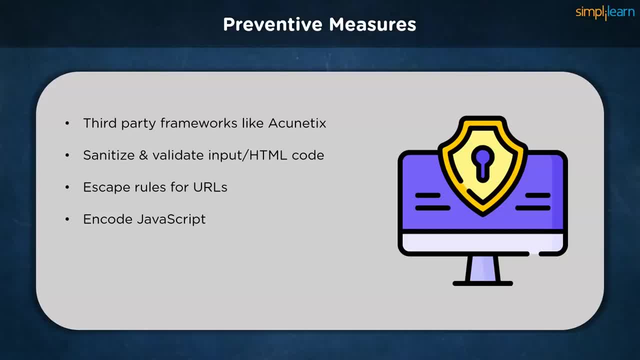 HTML context, So you need to first Unicode escape the input and then HTML encode it. Content Security Policy, or CSP, is a computer security standard introduced to prevent cross-site scripting, click-jacking and other code injection attacks resulting from the execution of malicious content in the. 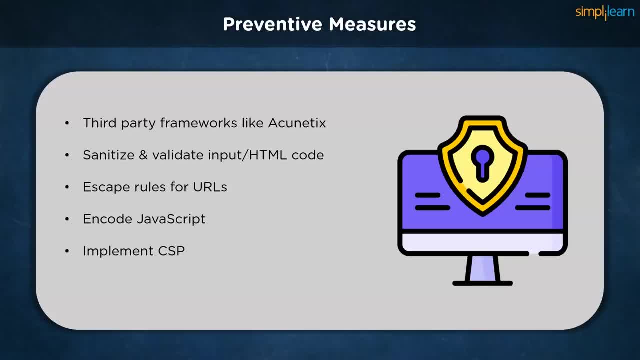 trusted web page context. It is a candidate recommendations of the W3C working group on web application security. It's widely supported by modern web browsers and provides a standard method for website owners to declare approved origins of content that browser should be allowed to load on. 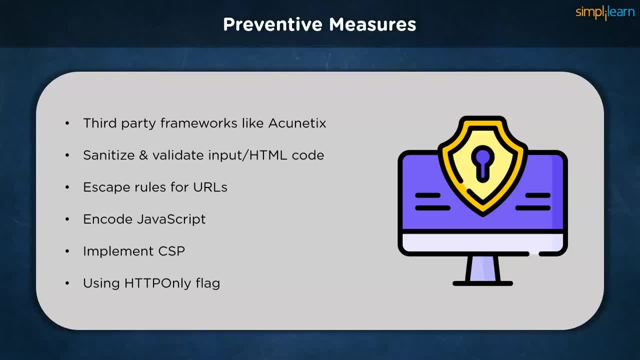 that website. HTTP only is an additional flag in WordPress. It is included in a set cookie HTTP response header. Using the HTTP only flag when generating a cookie helps mitigate the risk of client-side script accessing the protected cookie. that is, if the browser supports it, If the HTTP only flag. 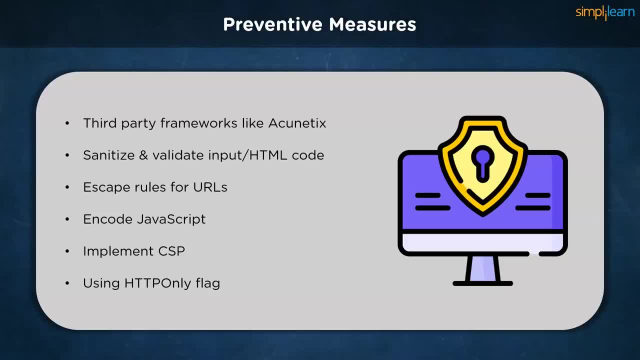 is included in the HTTP response header. the cookie cannot be accessed through a client-side script. Again, this is if the browser supports this flag. As a result, even if a cross-site scripting flaw exists and a user accidentally accesses a link that explains the flag, the user can't access the flag. The user can't access the. 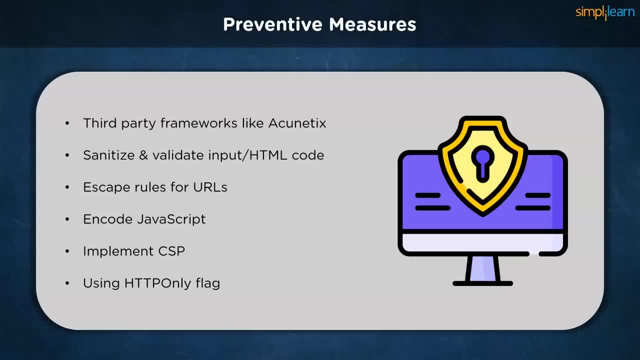 link. If a user exploits this flaw, the browser will not reveal the cookie to a third party. If a browser does not support HTTP only and a website attempts to set an HTTP only cookie, the HTTP only flag will be ignored by the browser, thus creating a traditional 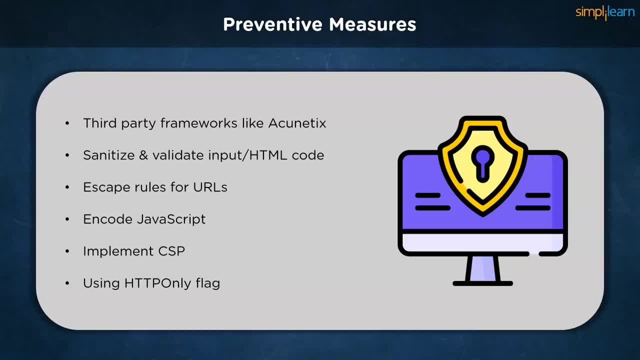 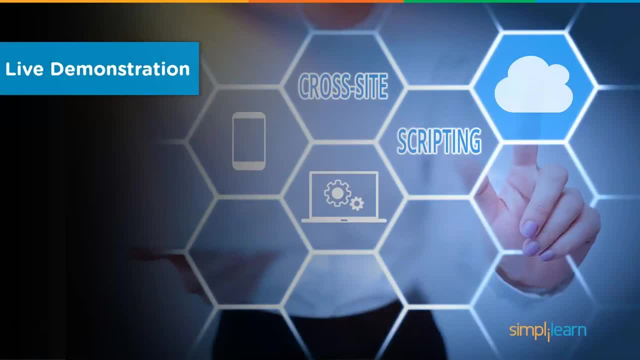 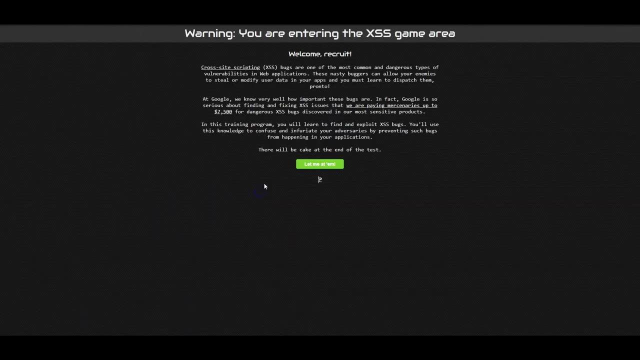 script accessible cookie. As a result, the cookie becomes vulnerable to theft of modification by any malicious script. Next on our docket is a live demonstration where we solve a set of cross-site scripting problems, starting from the basic level to the top-most level, 6. We're going to start. 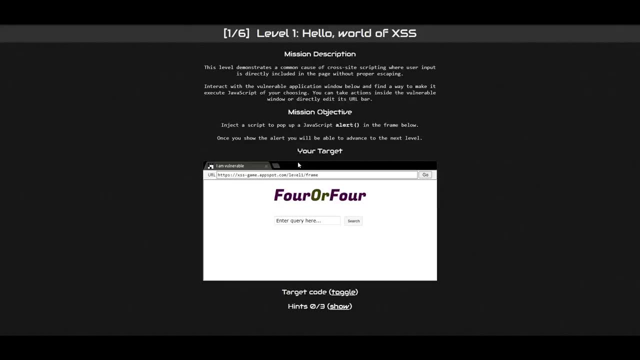 at level 1.. In this verb application it demonstrates the common cause of cross-site scripting, where user input is directly included in the page without proper escaping. If we interact with the vulnerable application window here and find a way to make it execute JavaScript of 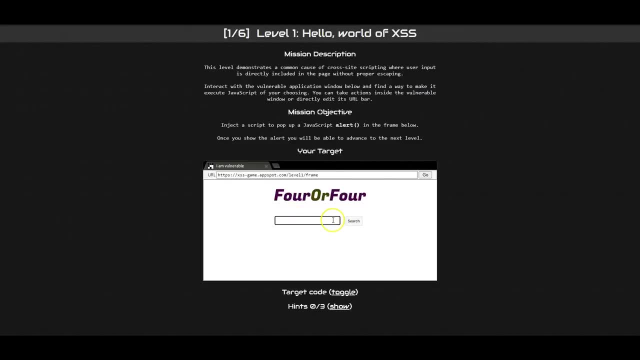 our choosing. we can take actions inside the vulnerable window or directly edit it into the URL bar. This task needs only basic knowledge. Let's see why the most primitive injections work here right away. Let's do a simple query and inspect the resulting HTML page. 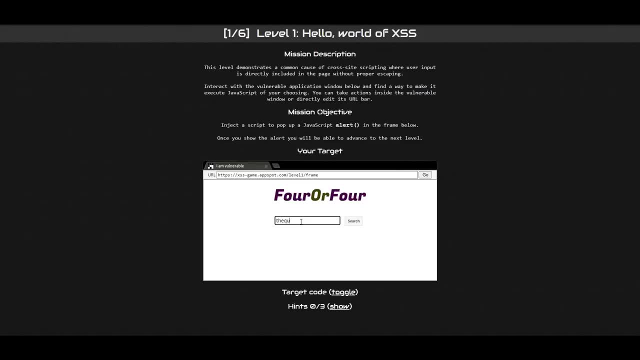 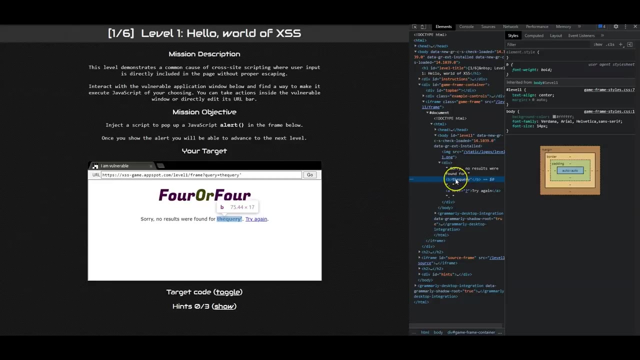 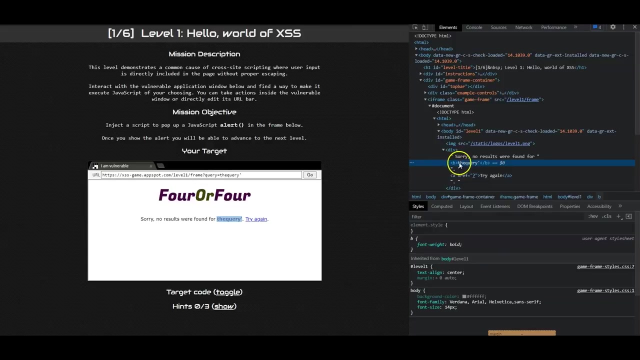 I'm going to use this phrase with a single quote as a special character. We can now inspect the HTML page. We can see here in this line, The special character single quote appears in the result over here. The provided query text is placed directly in a tag as in a body element. 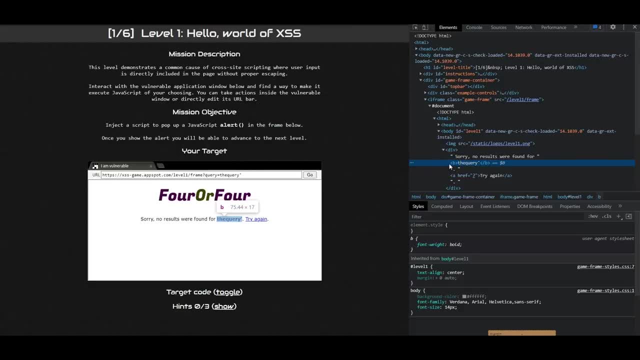 We need to perform a reflected XSS into the web application because they are non-persistent XSS attacks and the payload should be included in the URL to perform successive XSS attacks. We need to perform a reflected XSS into the web application because they are non-persistent. 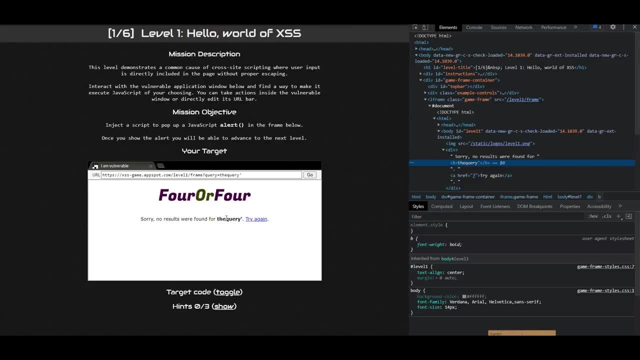 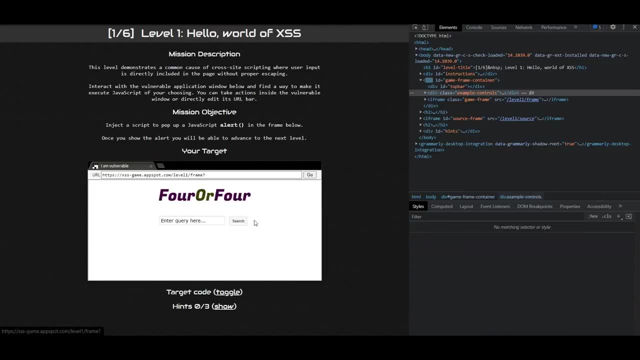 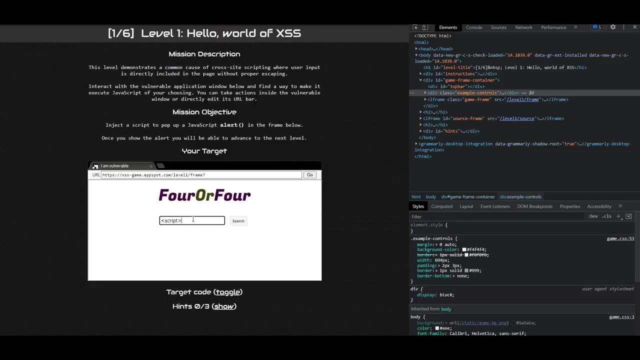 successful exploitation. We can use any payload, but we're going to use the simple one to perform an alert in this web application. It's simple and can be shown easily. We're just going to write the script over here And we're going to press search. As you can see, we have successfully. 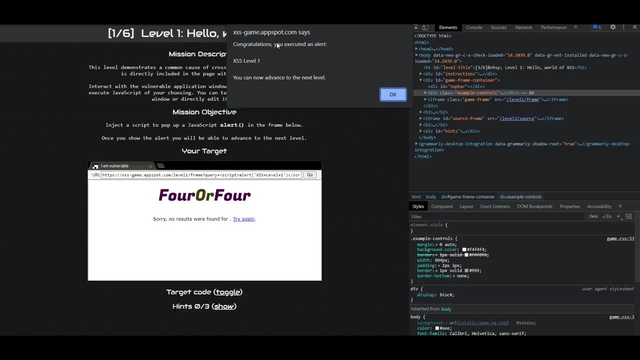 launched our first cross-site scripting attack. We can see an alert box pop up with the next script And we can see that we have successfully launched our first cross-site scripting attack. We can see an alert box pop up with the next script And we can see an alert box. 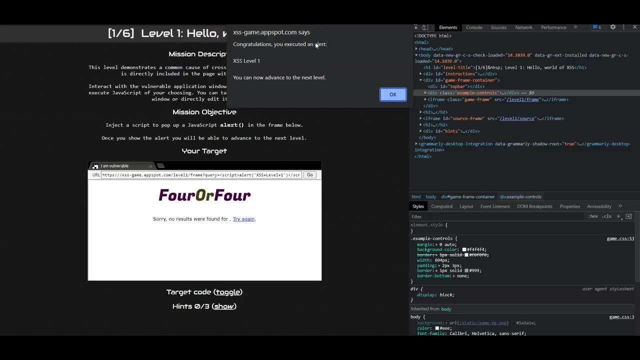 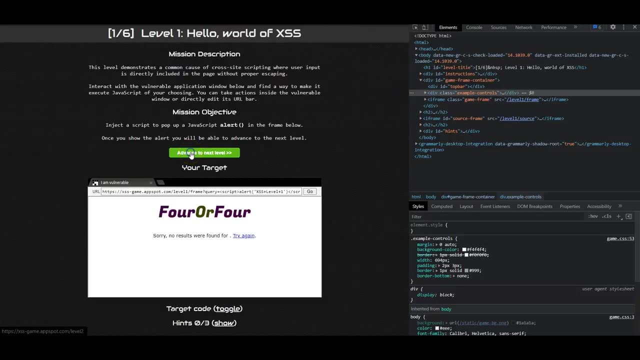 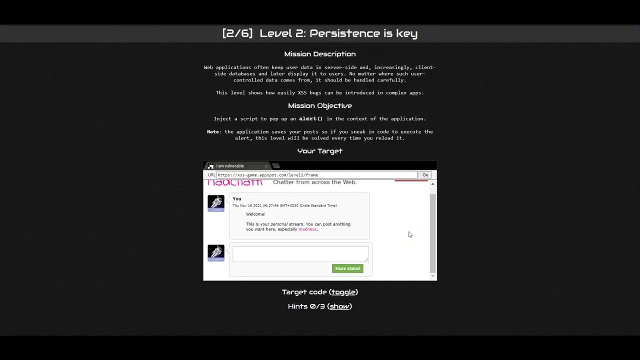 message And a similar process can be used to steal browser cookies and passwords, albeit with different commands. Now we have the option to move to level two In this web application. it shows that how easily XSS bugs can be introduced in complex chat applications. 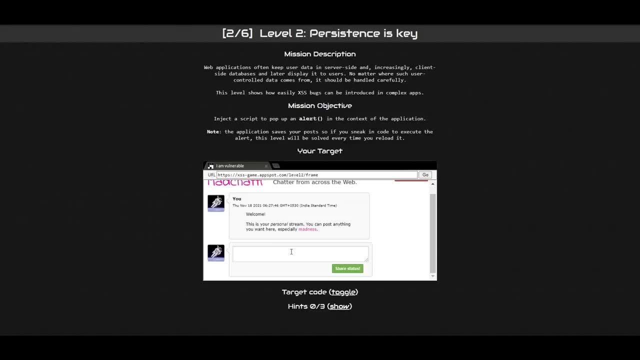 Chat app conversations are stored in a database and retrieved when a user wants to see the conversation. Therefore, if a malicious user injects some JavaScript code, all visitors will be infected. This kind of cross-site scripting attack is more powerful and it is more riskier than reflected cross-site scripting attacks, And that's why it's known as. 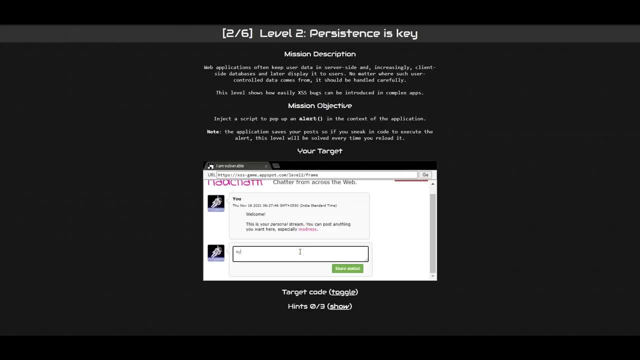 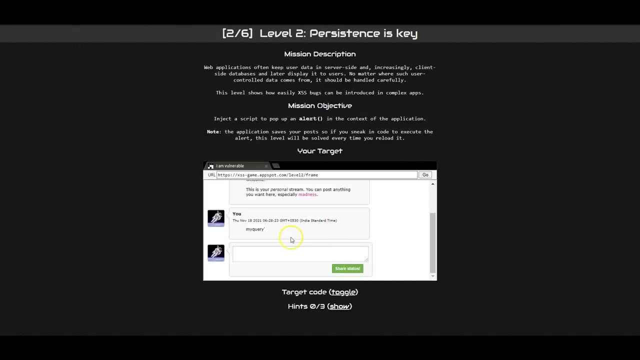 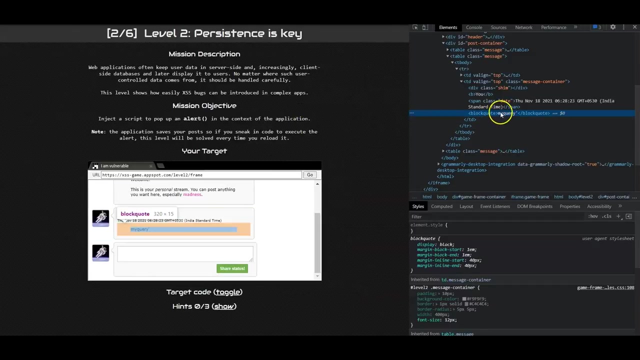 stored XSS. I posted my query with a special character of a single quote And this is what I get. Whatever I typed in simply appeared on the page right after I click on share status. Let's see the source. You can see here the text I posted seems directly put inside a block code tag. So even a simple 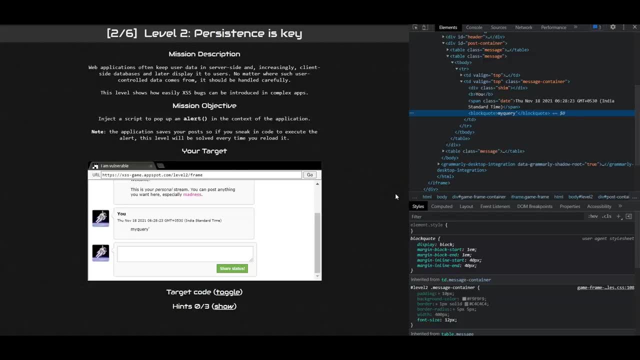 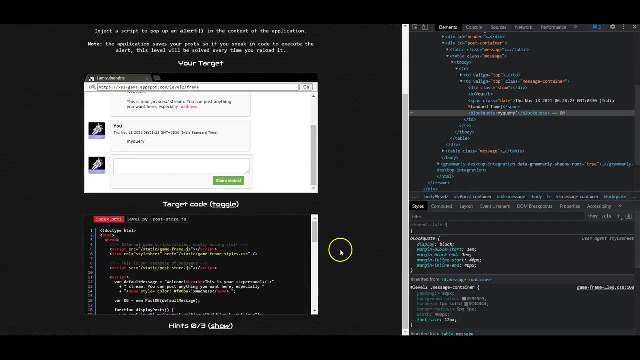 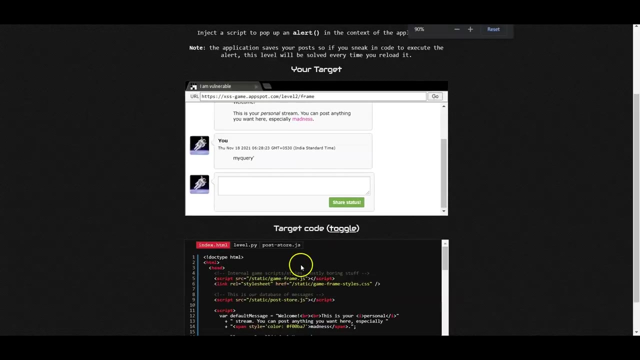 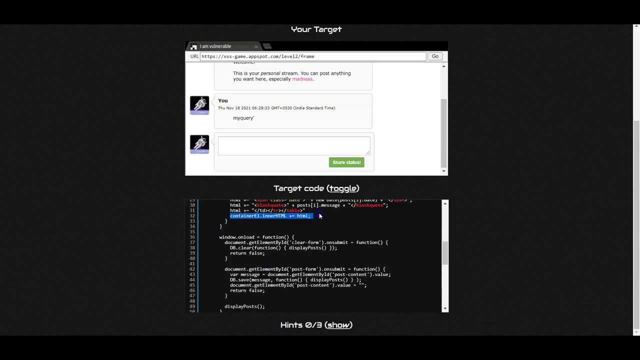 script tag we used in level one should work here, but it will not. Let us examine the code to understand why. We're going to toggle the code away here and check the indexhtml file. Important part is line 32.. The generated HTML fragment, which is the HTML variable in the code. 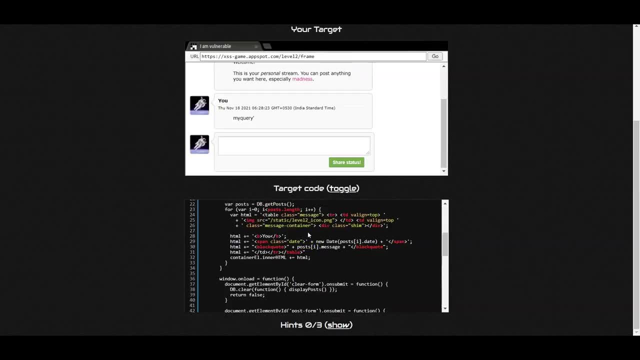 is added to the mail HTML using the inner HTML method. So when the browser parsing this HTML fragment, it will not execute any script tag defined within that HTML fragment. HTML parser will not execute a script tag when it parses HTMLs via the HTML tag. So when the browser parses this, 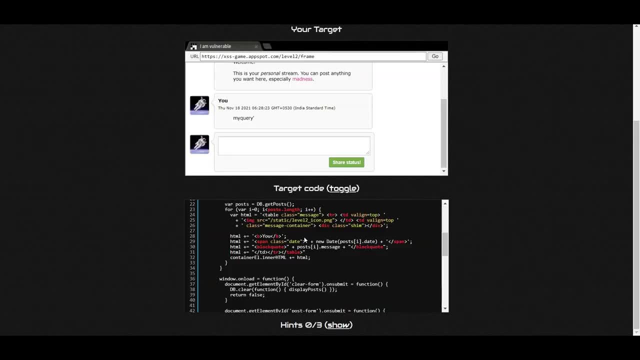 HTML fragment. it will not execute any script tag inside this method. This is why the script tag, like we used in level one, is not going to work here. Our solution is to use events. Events will execute the defined JavaScript. We're going to use an image over here. 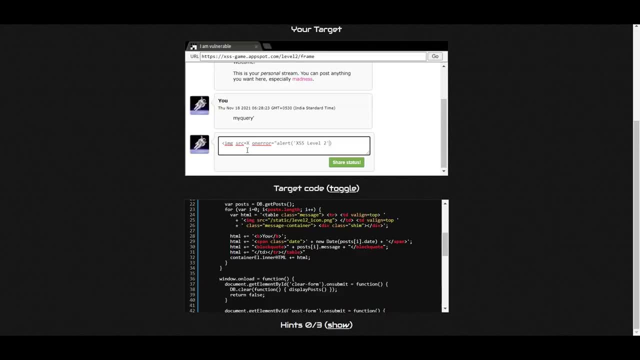 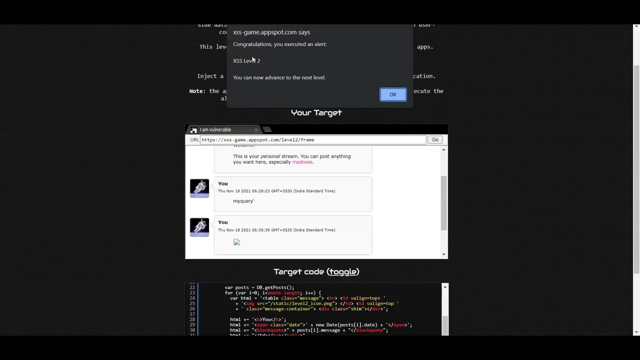 And when we press on share status in the above injection, we are loading an image that doesn't exist, which causes to trigger an onError event. In onError event it will execute our alert method. With that we are able to beat level two and we can now move up to the next level in 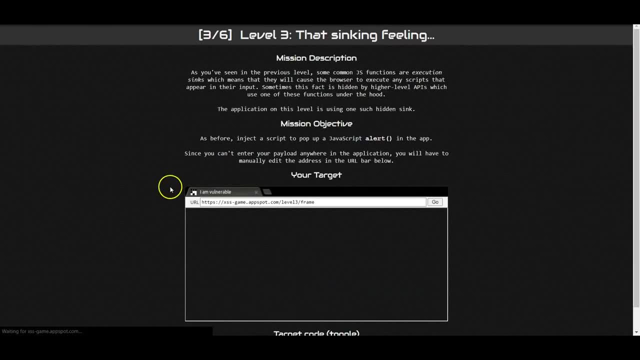 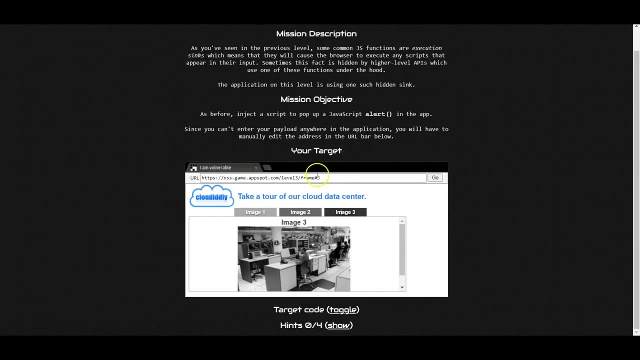 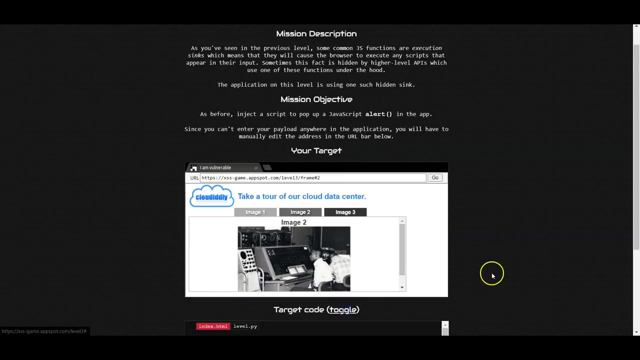 our challenge. As you can see, clicking on any tab causes the tab number to be displayed in the URL fragment. This hints that the value after the hashtag controls the behavior of the page. That is, it is an input variable. To confirm, let's analyze the code. 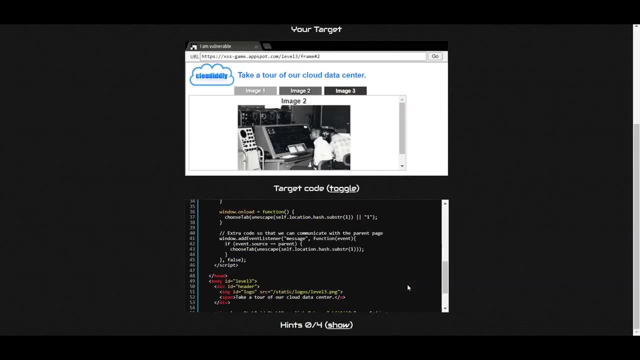 As you can see in line 43,, inside the event handling, the value provided after the hash in the URL is directly passed onto the true tab method. No input validation is being performed. The value passed to the choose tab method is directly injected into the IMG tag in line. 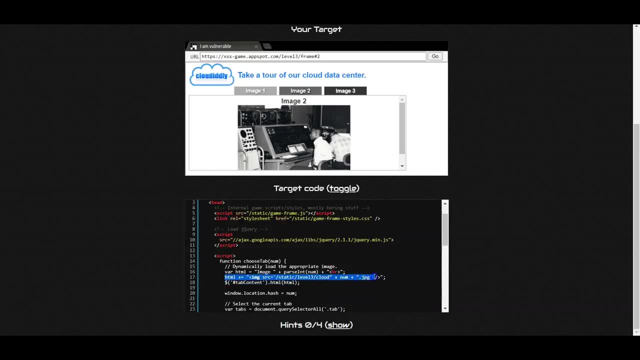 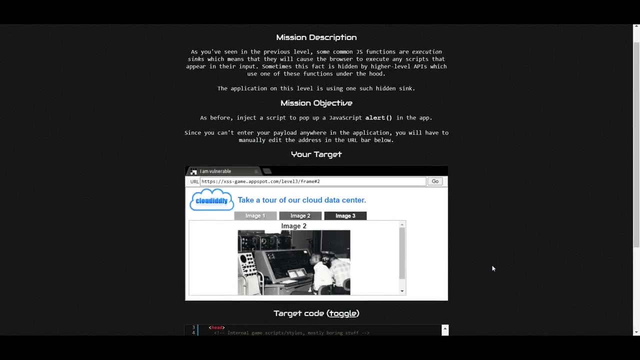 17.. This is an unsafe assignment and it is the vulnerable part of the code. Now. all we have to do now is to craft a payload that would adjust the IMG tag to execute our JavaScript. Remember, the script tag from level one would not work here, since the variable HTML is. 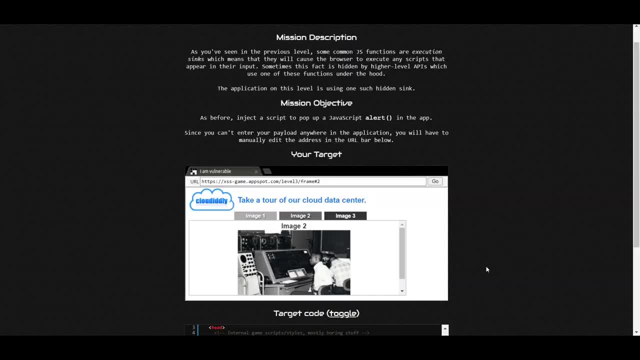 used to add the DOM dynamically, hence the events are our aces here. once again, I will choose to use the existing IMG tag and change the source to something that doesn't exist. I am forcing it to fall in to execute an onError, even which I will pass the URL. 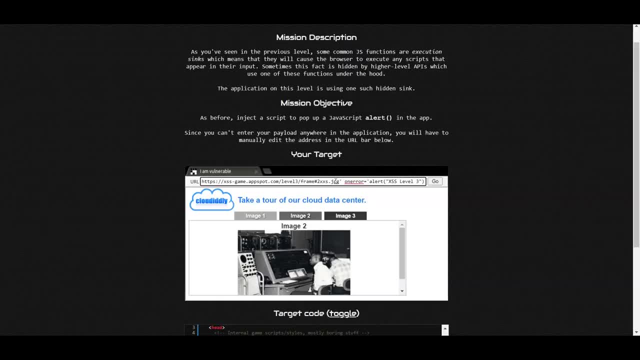 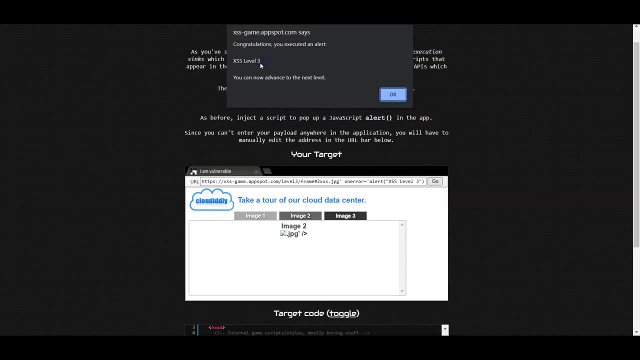 Once we visit that URL, we can see that our java popup has opened up here with the same message of XSS. level 3 has been completed With this. we can now move on to level 4, which is going to present a different kind. 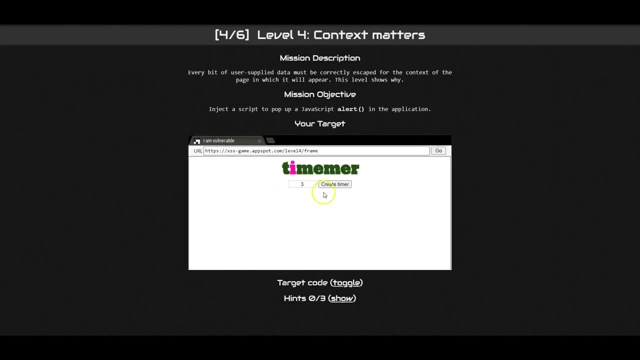 of attack. In this server application, there is a timer on the page. This is a timer that is used to set the time of the attack. In this server application, there is a timer on the page that is used to set the time of. 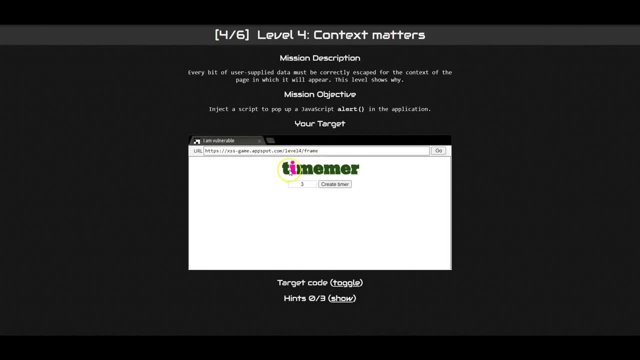 the attack. In this server application there is also a timer on the page that is used to set the time of the attack. That means, whatever numbers we put in the box, a countdown starts and then, when it finishes, the application alerts that the countdown is finished. 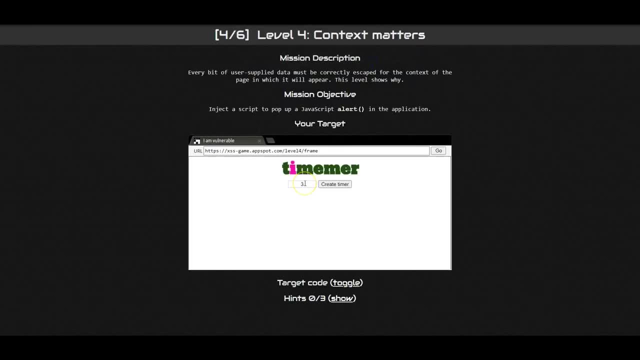 And we can see the timer is a popup appearing over here and this resets the timer again. Now it is obvious that the value entered in the text box is transferred to the server over the timer parameter in the URL. Let us examine the code to see how the timer parameter works. 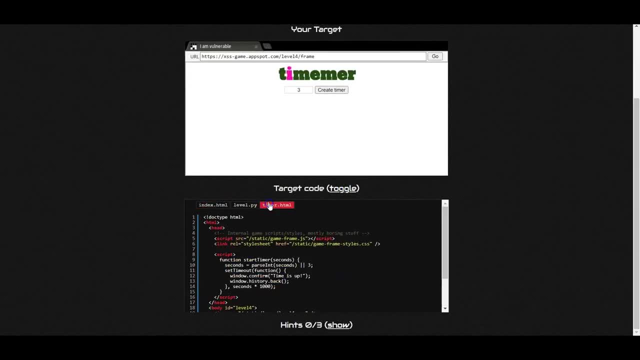 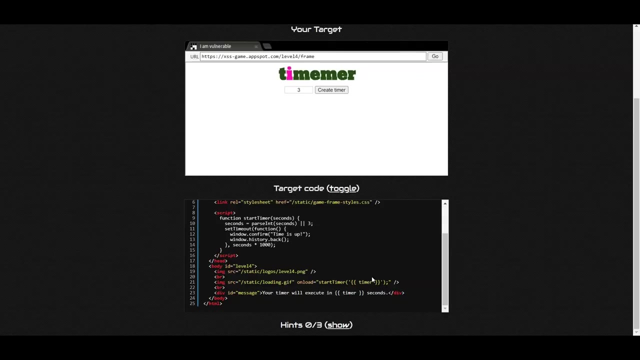 is being handled. we're going to visit timer dot HTML over here and we're going to check over here. in line 21, the start timer method is being called in the onLoad event. however, the timer parameter is being directly passed to the start timer method. we need to perform a pop-up alert in the web application, which 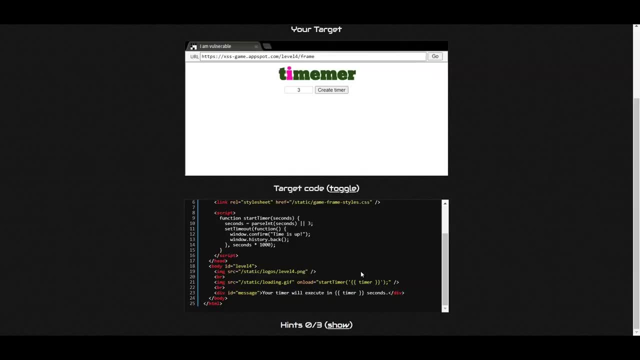 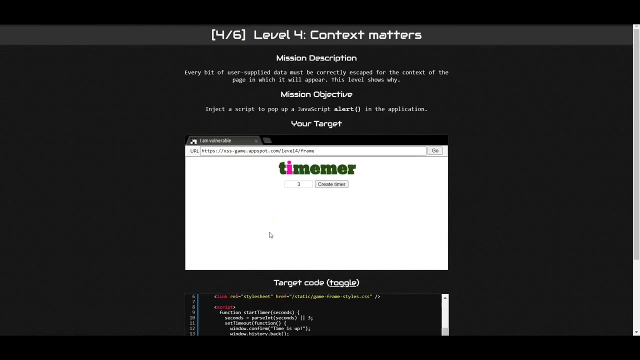 escapes the content of the function start timer without baking the JavaScript code. the parameter value is directly added to the start timer method without any filtering. but we can try to do here is to inject an alert function to be executed inside the onLoad event along with the start timer. 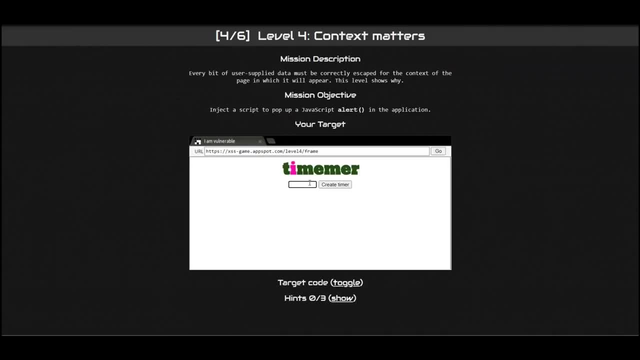 method. we're going to remove this argument and put our script over here. now I may press on create timer and we have a pop-up with the XSS level 4 completed. we can now move on to level 5 in this web application. this application, XSS, is different because this: 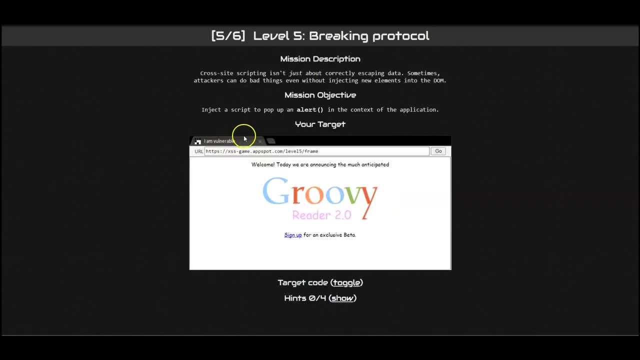 challenge description says cross-site scripting isn't just about correctly escaping data. sometimes attackers can do bad things even without injecting the new elements into the DOM. it's kind of open redirect, because the attack payload is executed as a result of modifying the DOM environment in the victims browser. this environment is used by the original client-side script, so 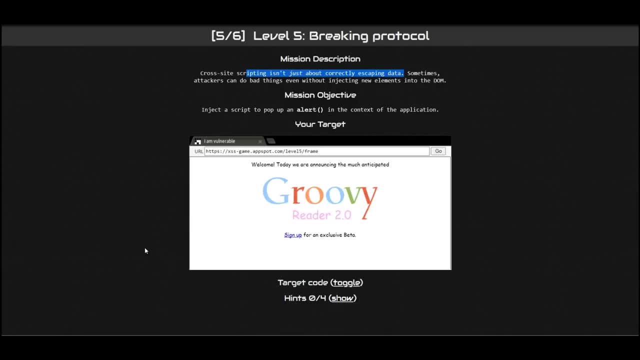 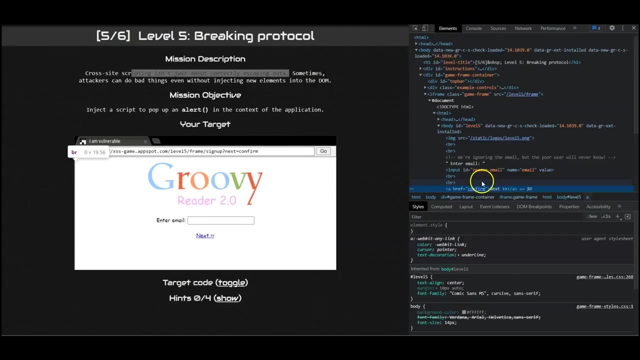 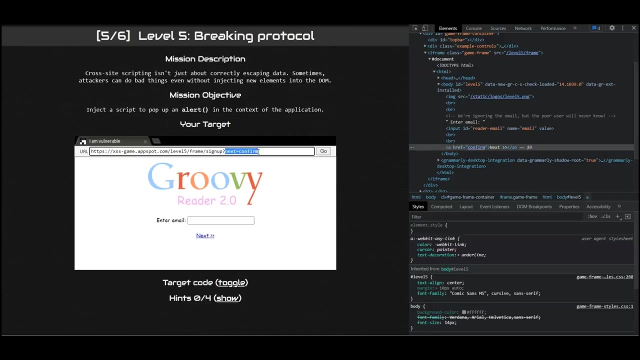 that the client-side code runs in an unexpected manner. the vulnerability can be easily detected if the next link in the signup page is inspected. the HREF attribute value of next link is confirm, which is exactly the value of the next URL query parameter. as you can see over here, this means using the next. 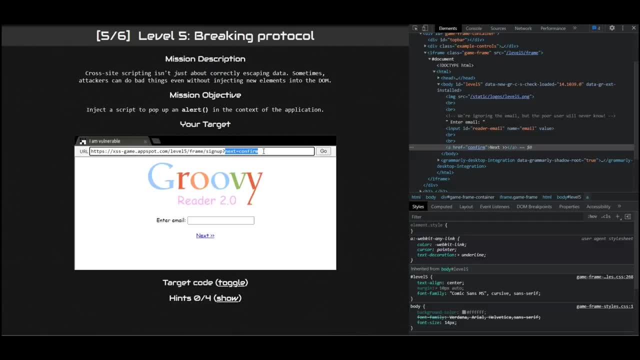 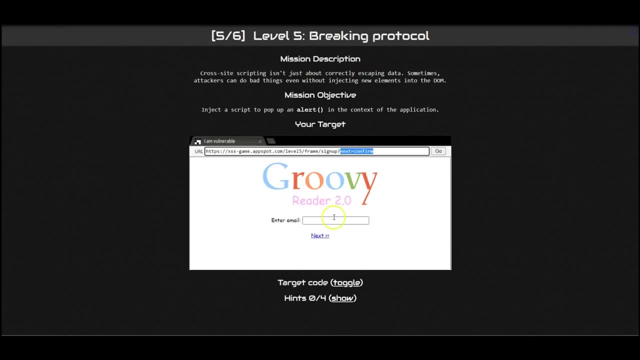 query parameter can be used to inject a JavaScript code to the HREF attribute of the next link. the following is the best way to do it: as soon as the user clicks on the link, the script will be triggered. we're going to press anything random. we're going to press anything random. 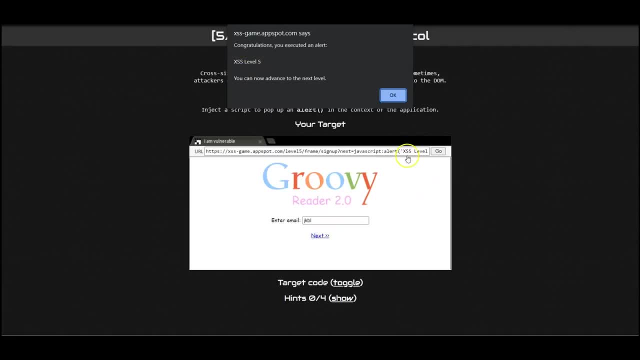 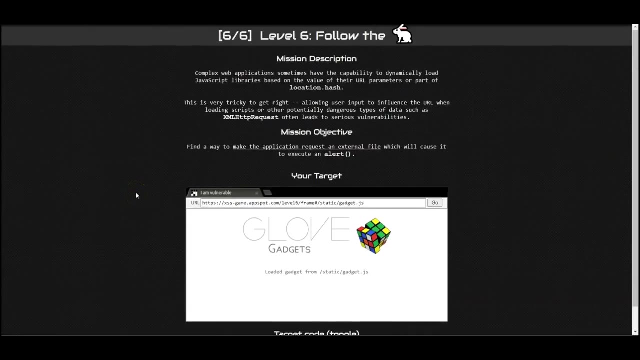 and now that we click next, we can see the XSS level 5 that we had provided in the URL as a parameter to the next variable. since the value of next provided appears on a pop-up, we can consider the attacker success and move on to the final level 6 in this server application. it shows some of the 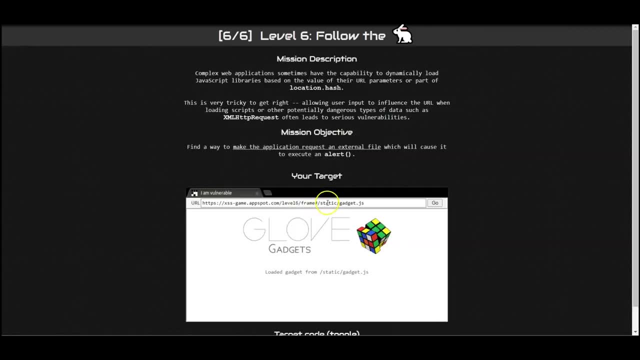 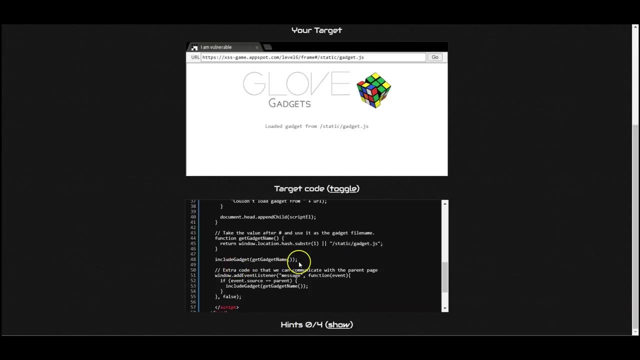 external JavaScript is retrieved. if you analyze the URL, you can see that the script is loaded already. the vulnerability lies within the script, inside the script, and the API is also in the script as well, and the HREF category allows us to change the URL yourself and the HTML, the URL itself. 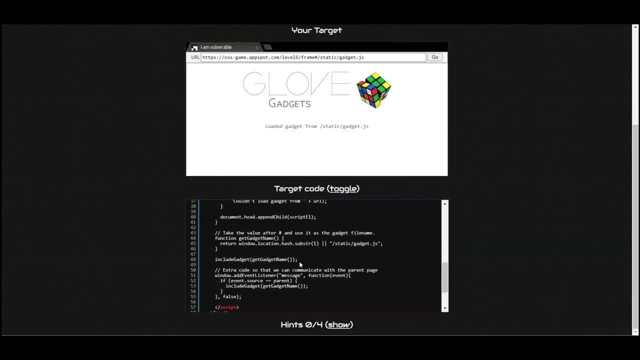 is in the kindle and the HREF category as well and we can check it out here. for example, there is the number of the pieces and the name of the piece is actually the ID, so of the piece is a value in the HREF category and we can. 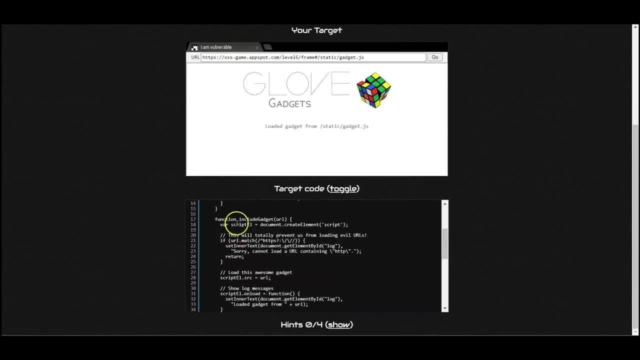 see that the value of the piece is not necessarily the same as the value of the else that we have created, so we are going to take a look at that and fix it. A script tag is created and the URL gadget name parameter value is directly used as the. 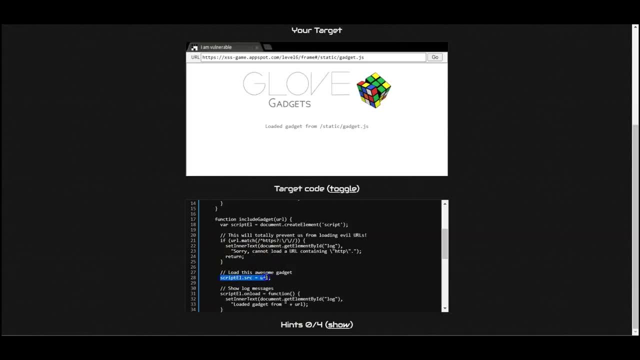 source attribute of the script tag in line 28.. This means we can completely control the source attribute of the script tag that is being created. That is, with this vulnerability, we can inject our own JavaScript file into the code. We can inject a URL of our own hosted JavaScript into the web application's URL after the: